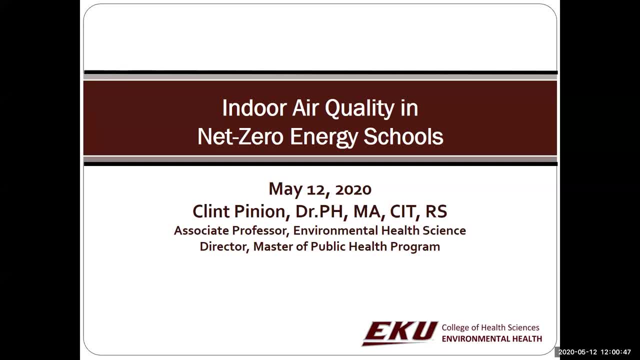 Organization of Work Factors Associated with Workability Among Aging Nurses. as a part of our NIOSH ERC Ergonomics Webinar Series. On June 3rd we'll be joined by Suzanne Turan from UC Berkeley's Labor and Occupational Health Program. 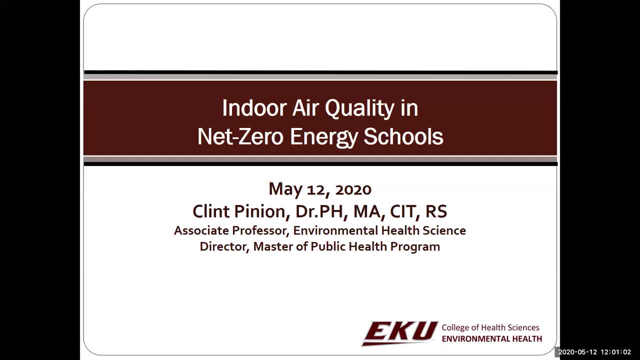 Kevin Riley from UCLA's Labor Occupational Safety and Health Program and Teresa Andrews from UC Davis Western Center for Agricultural Health and Safety for a free webinar on protecting California workers from wildfire smoke. Our next NIOSH ERC Industrial Hygiene Webinar will be on June 9th with Dr Elizabeth Knoth and Dr Kathy Hammond. 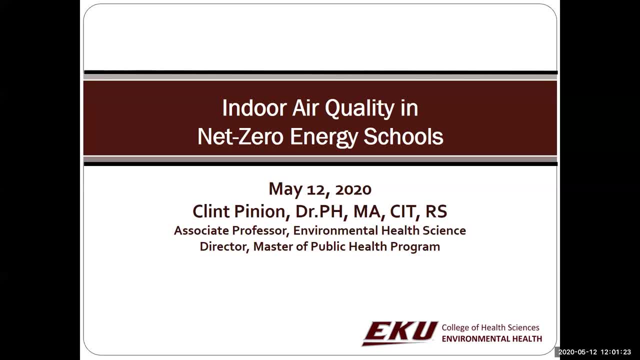 on Exposure Assessment for Epidemiology Risk. This webinar will be focused on the use of routine industrial monitoring data. For more about these upcoming events, you can visit coehberkeleyedu backslash about CE And on behalf of the NIOSH-supported education and research centers throughout the country. 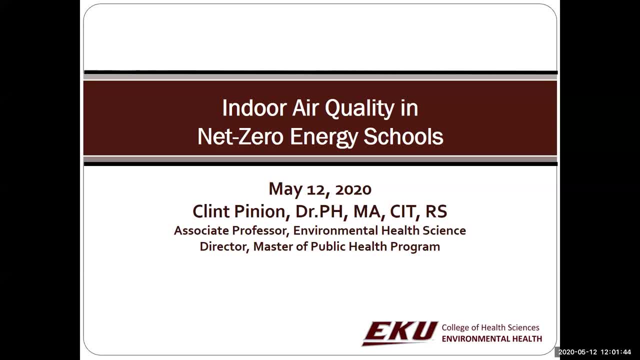 we're pleased to present the 2020 Industrial Hygiene Webinar Series, offering free webinars the second Tuesday of each month. This collaborative effort, on behalf of each ERC's continuing education program, aspires to provide access to current research supported through NIOSH ERC programs. 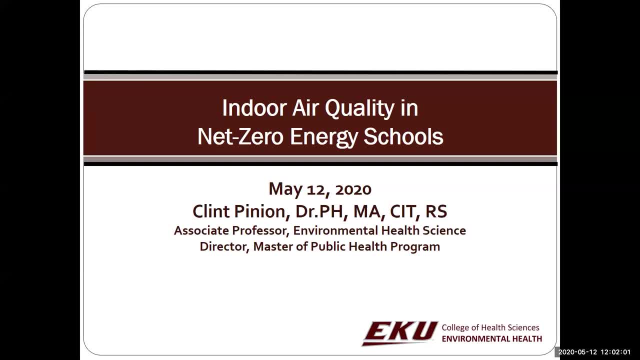 Thank you so much for joining us. Today's webinar Indoor Air Quality in Net Zero Energy Schools is brought to you by the Central Appalachian Regional Education and Research Center and Dr Clint Pinion. A few housekeeping items first. You will be muted during this presentation. 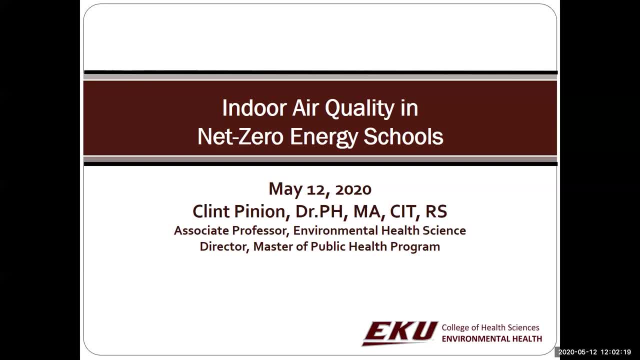 If you would like to ask a question, please enter it into the online Q&A. We will save time at the end of this presentation to address all questions. As a reminder, participants who have logged in with their registration email for the full live presentation today. 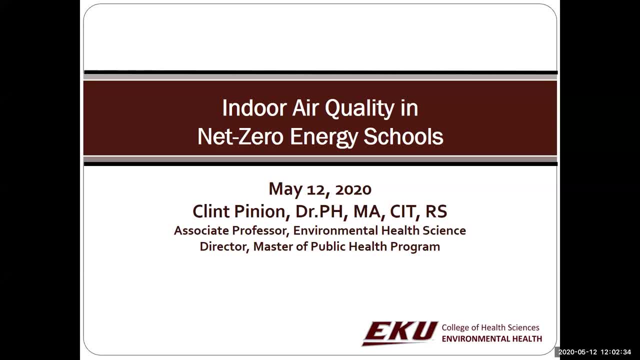 will receive a link to the recording and an evaluation form that will qualify participants for certificate of completion with one continuing education contact hour. Once you complete this online evaluation, you'll be able to access your certificate. This email will come to you tomorrow roughly the same time tomorrow around noon. 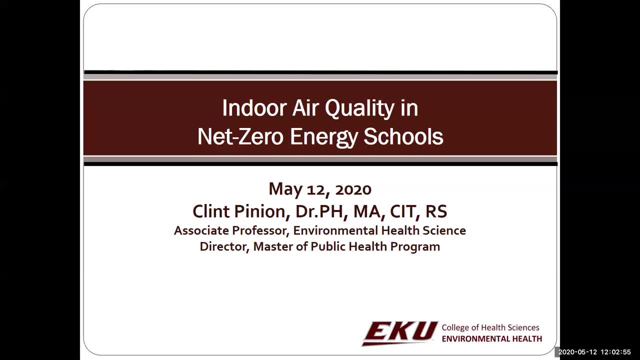 This presentation is being recorded and will be made available on the COEH Northern California's YouTube page and on our website At this time. we're pleased to welcome our presenter. Dr Clint Pinion is Associate Professor in the Department of Environmental Health Science. 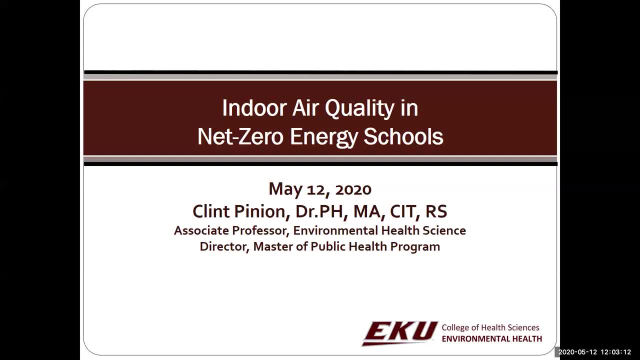 and Director of the Master of Public Health Program at Eastern Kentucky University. He spent six years as a health, safety and environmental professional in the oil and gas industry in the Houston area, serving in roles such as the global health, safety and environmental education and training manager. 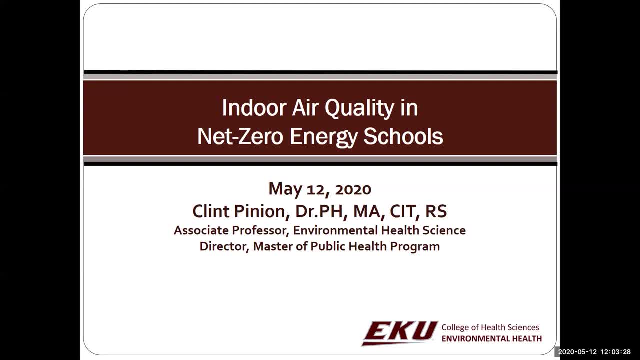 and environmental technician for a global engineering, procurement, fabrication and construction company. He currently serves as a consultant for an environmental and occupational health consulting group based in Lexington, Kentucky. Dr Pinion earned his Doctor of Public Health degree in Environmental and Occupational Health Science. 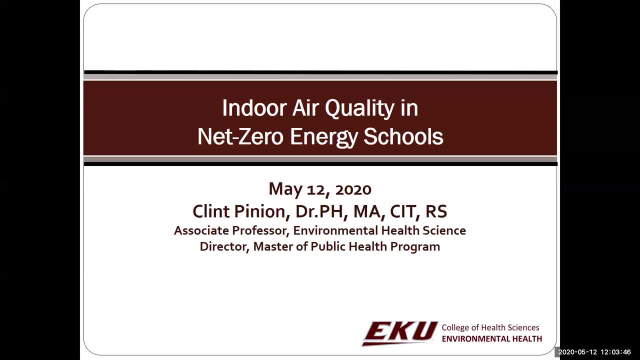 from the University of Texas Health Science Center at Houston UT Health School of Public Health. He also earned a Master's of Public Health degree and Master's of Arts in Higher Education from Eastern Kentucky University and a Bachelor of Arts degree in Biology from Berea College. 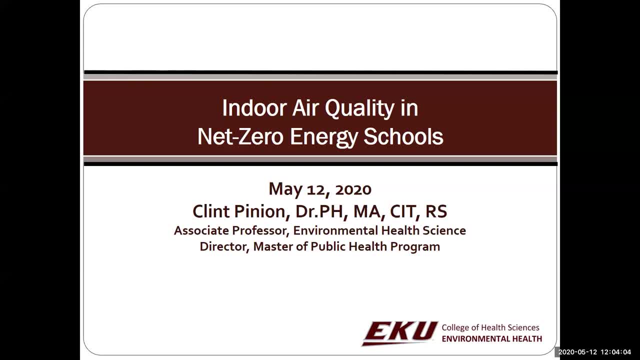 He currently serves as President of the American Industrial Hygiene Association Kentuckiana Section, past President of the Association of Environmental Health Academic Programs and President-Elect of Kentucky Environmental Health Association. Dr Pinion is a registered sanitarian in the Commonwealth of Kentucky. 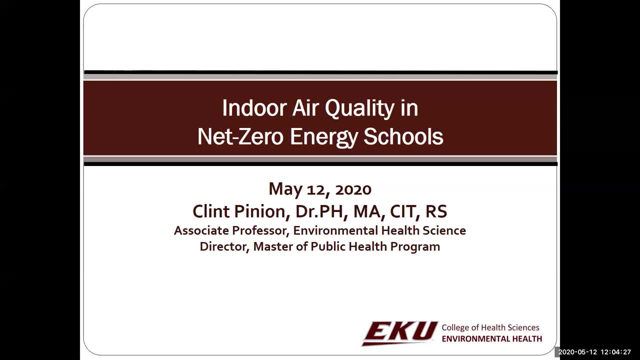 and a certified instructional trainer through the Board of Certified Safety Professionals. He received the EKU Creative and Critical Thinking Teacher of the Year Award in 2017 and 2019.. Thank you so much for joining us, Dr Pinion. Thanks for having me. 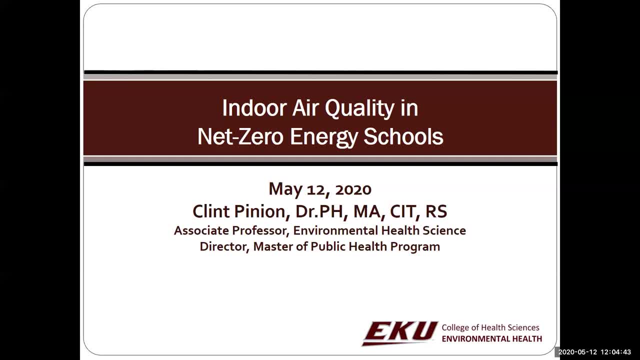 It's a pleasure, I'll go ahead and get started. Thanks for everyone for joining today. This presentation will be based on a consulting gig, if you will, that one of my colleagues and I completed in the Midwestern portion of the United States. 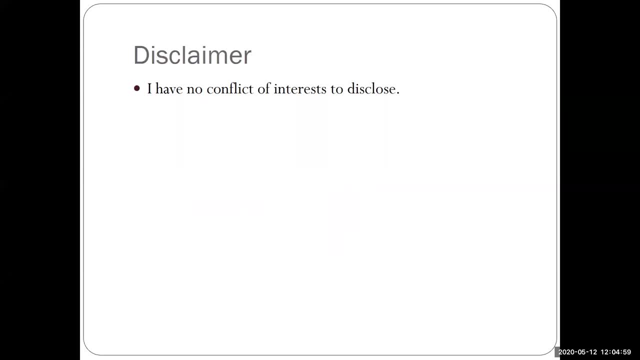 And before I begin, I just wanted to give a disclaimer that I have no conflict of interest to disclose to you Now. many of you may already know what we're going to go over in terms of the content, but hopefully you'll take away something new today. 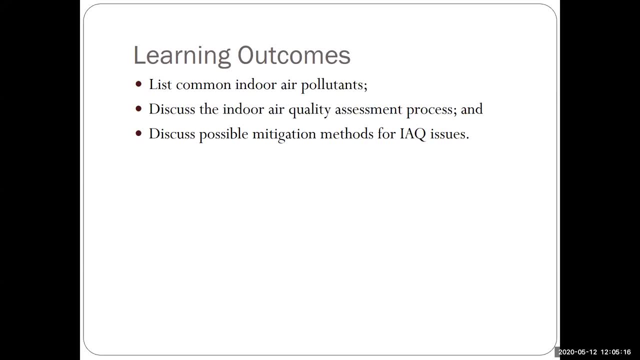 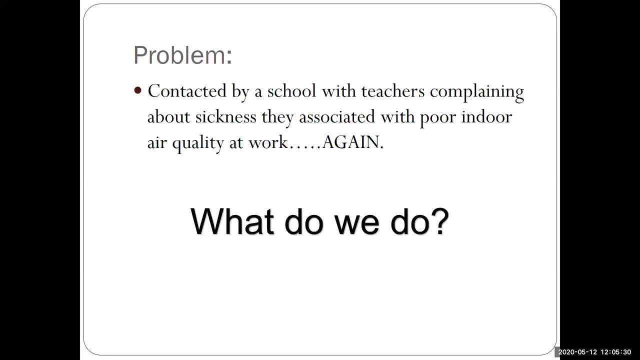 The learning outcomes for you, though, just in case you missed it on the flyer- is to list common indoor air pollutants, discuss the indoor air pollution, the indoor air quality assessment process and discuss possible mitigation methods for indoor air quality issues. So, as many of you probably have experienced, 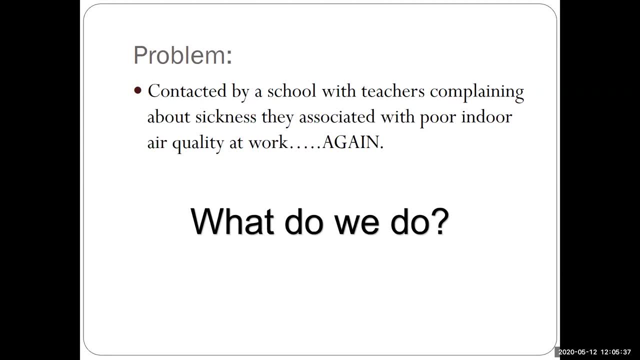 in your careers as a consultant, as an academic, folks come to you when they see that you work in environmental and occupational health with you know very strange and then sometimes very mundane issues. So a colleague and I were contacted by a school. 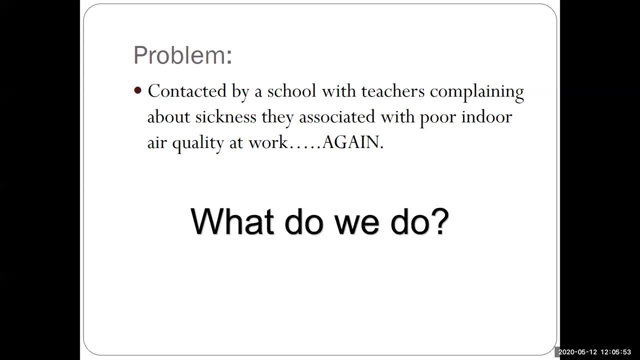 in the Midwestern portion of the United States and they had teachers that complained about being sick, And the teachers believed that the sickness they were experiencing was associated with poor indoor air quality at their work. Now just for a few points of emphasis. 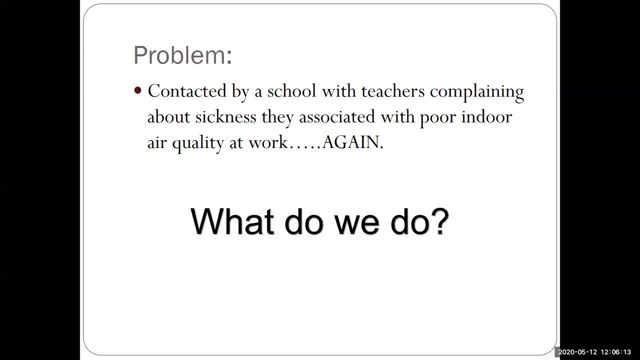 this school had undergone several IAQ studies in the past and all the readings would come back normal, but the teachers would still have the same complaints: They were drowsy, they were experiencing headaches, stuffy nose, irritated throat- many of the symptoms that you would associate with IAQ. 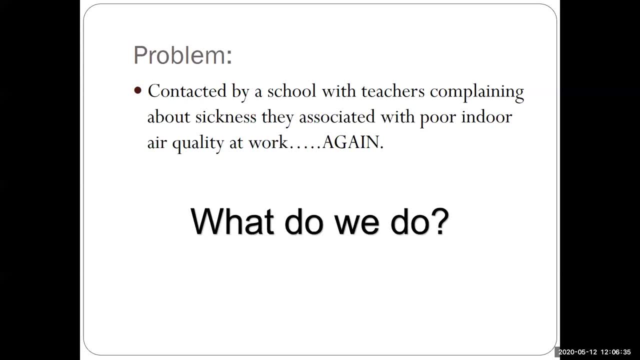 but also many of the same symptoms you would associate with the common cold. So a little background about this school. They are a net zero energy school, which means essentially that they will not take more from the grid than they actually can put back. So if you think about it, 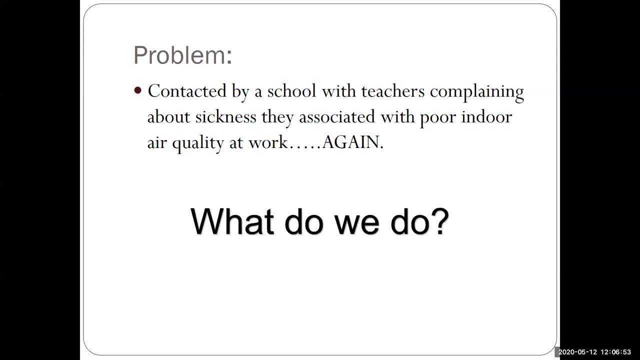 when you have a zero net energy consumption school, the total amount of energy used by that building on an annual basis is equal to the amount of renewable energy that's created on that site, And so this school was established in 2011,, and really the whole focus of the design. 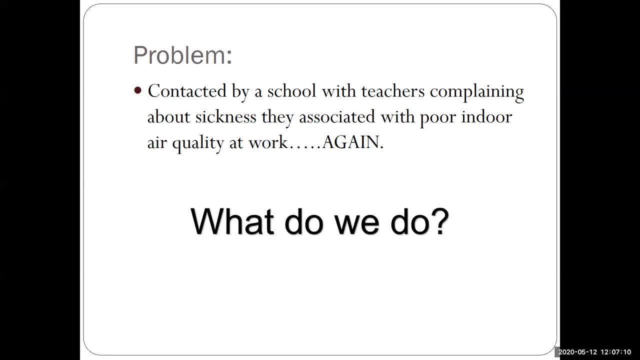 was that it was going to be energy and environmentally efficient. It has spacious classrooms with lots of labs. it has an equine program. it has a diesel engine program. that's all geared towards agriculture. They have their own aquaculture area for raising fish. 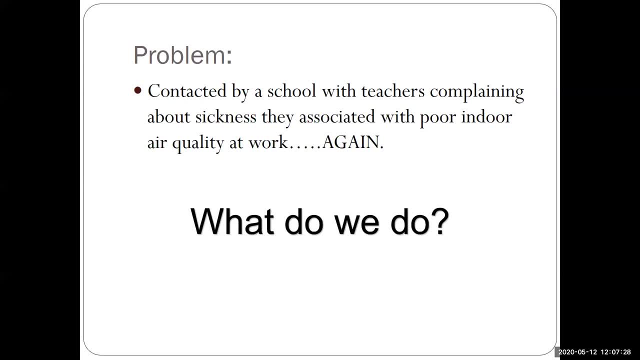 they have a huge auditorium for selling livestock. It's basically a dream school for anyone that's involved in agriculture. It's also a magnet school, meaning that students do not spend the entire day there, but of course the teachers do. This particular school uses solar panels. 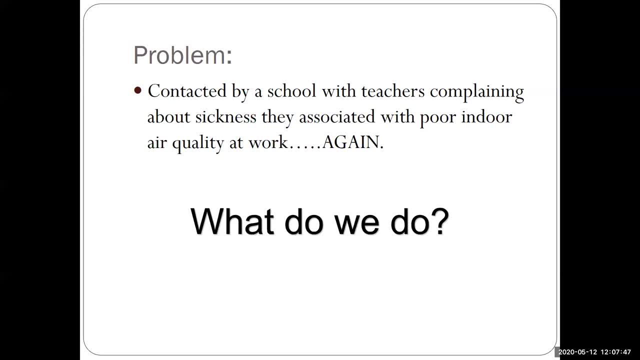 it has waste disposal through its constructed wetlands. it has rainwater collection systems that are built into the school building but also built into the barns and the arena, and they use that water for crop irrigation. So overall it's a very energy efficient school. 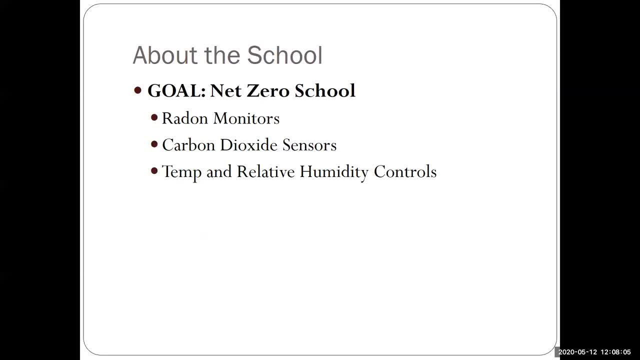 A few of the other items that were interesting about the school is that when it was initially built because of the location, they included radon monitors. They went ahead because it was state of the art, they wanted to be mindful of industry, they wanted to be mindful of indoor air quality issues. 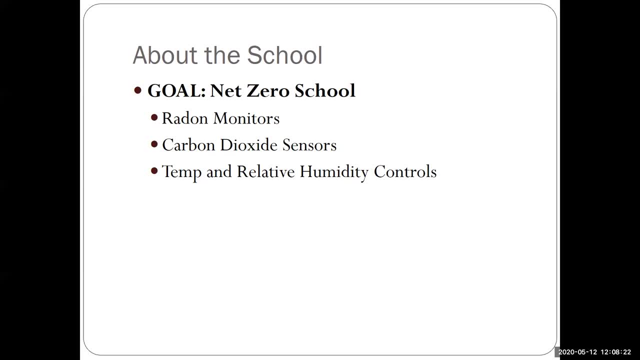 They actually had carbon dioxide sensors built into the school. And another thing, of course, with a lot of modern schools, they were able to control the temperature and relative humidity controls, which was, you know, for us. we're thinking: how do you have an indoor air quality issue? 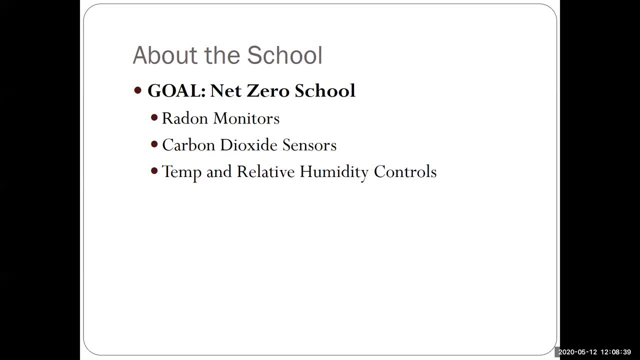 And so it really did raise the question for my colleague and I: what do we do? They've already experienced several different industrial hygienists coming in and doing IAQ studies. They come back with positive results, saying everything is fine. yet these teachers are complaining. 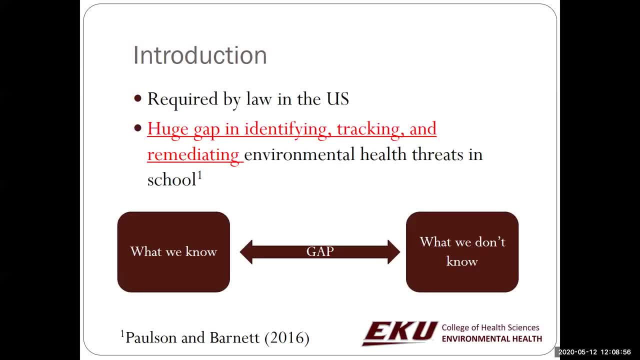 of the same issues. So I wouldn't be an academic if I didn't provide a little literature review. If you look at the literature that's available on indoor air quality issues, on the primary and secondary level of education, you will see that there's a huge gap. 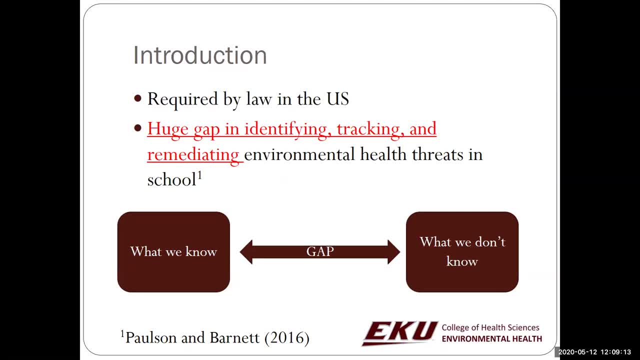 There's a large gap in identifying, tracking and remediating environmental health threats in schools. We know what we know, but we really don't know what we don't know And, unlike a lot of other places like work, you can choose to not work in a particular building. 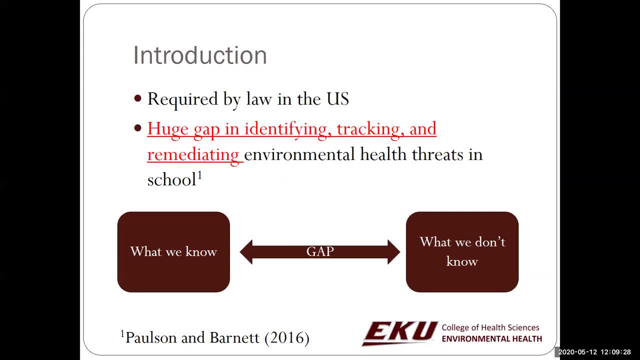 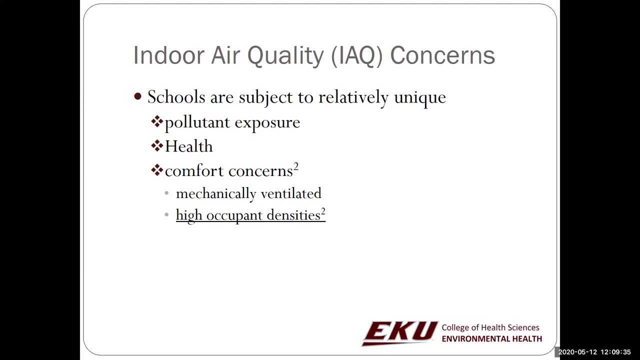 kids have to go to school at least from K through 12.. And because we have a lot of little bodies in small rooms- and there's more bodies these days, you know- sometimes up to 30 students in a classroom. you have high occupant densities. 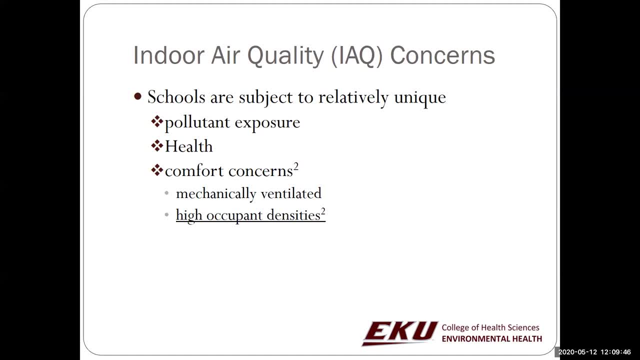 that are basically setting us up for more issues with IQ. So, higher levels of CO2, you know higher levels of CO, you will see those rise as we have more bodies in these rooms. You also set yourself up for other health issues. 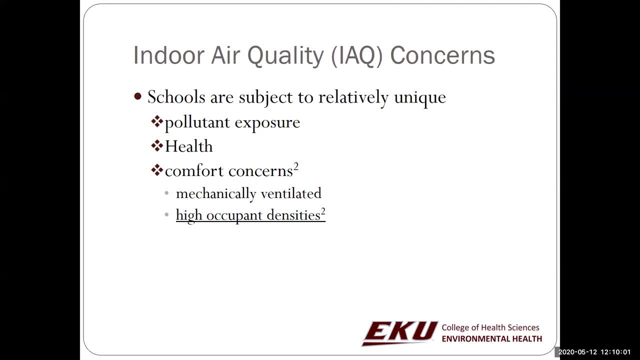 Think about passing communicable diseases. you know, like influenza through a school, It's going to go quickly because of how many people you're putting in such a small space. One of the things that we do look at, though, is these days. 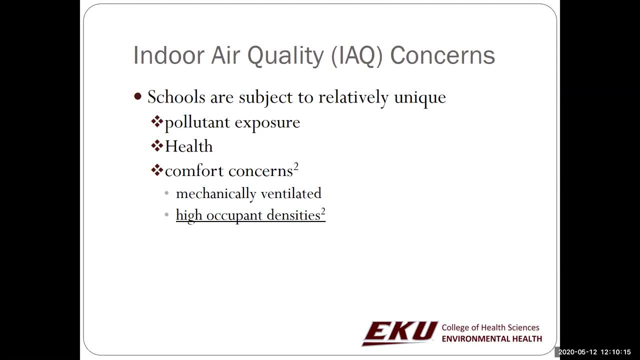 unlike when I was going to grade school. you know, most of the air exchange is mechanically ventilated. When I went to school we had windows, we opened them and we had natural ventilation. but most schools these days they go away from that. 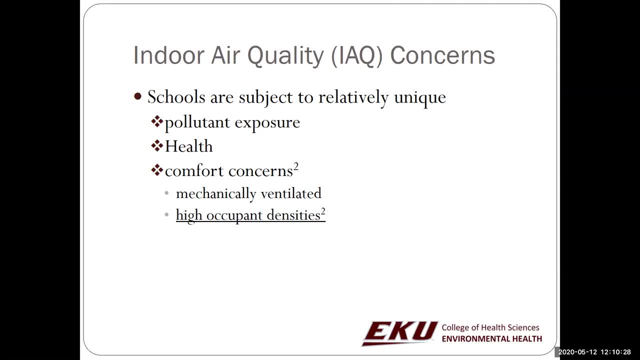 So you kind of put all of your faith into this system and if it's not working properly, you start to see IQ issues, indoor air quality issues. So some of the things we have to think about when we're going in to do an indoor air quality study. 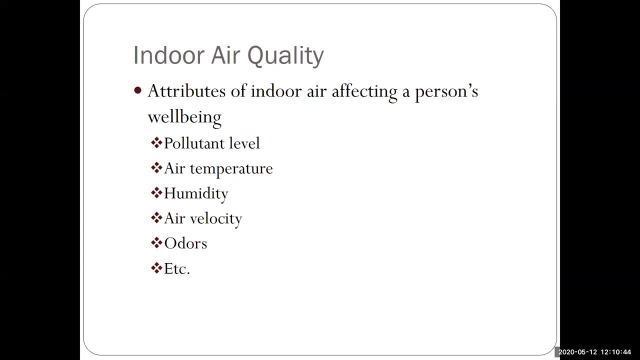 are the different attributes of the pollutants that are going to affect a person's wellbeing, And a lot of times we think about gases, we think about particulate matter, but we also have to think about some of those comfort parameters. Think about air temperature. 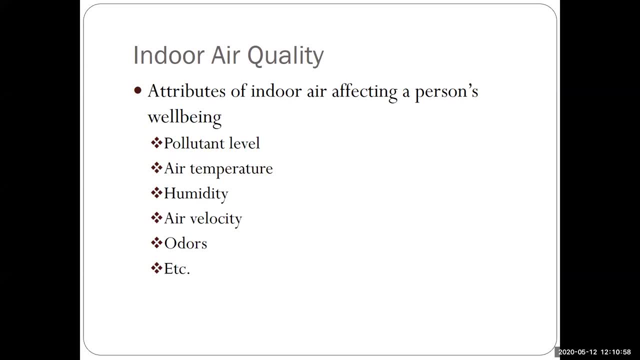 If you are uncomfortable, you are probably not going to perform at your optimal level. That's going to be the same thing for students. They're not going to academically perform well if they're not comfortable. Think about humidity: If it's too low, we're going to have issues. 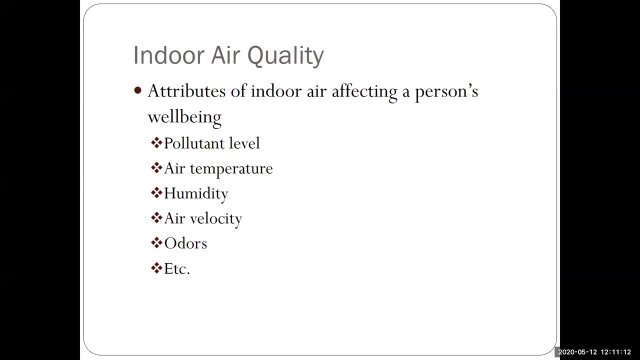 but if it's too high, we're also going to have issues. It's kind of like thinking about Goldilocks and the Three Bears. It's just right and that's what we're looking for. The air velocity: What's the exchange rate? 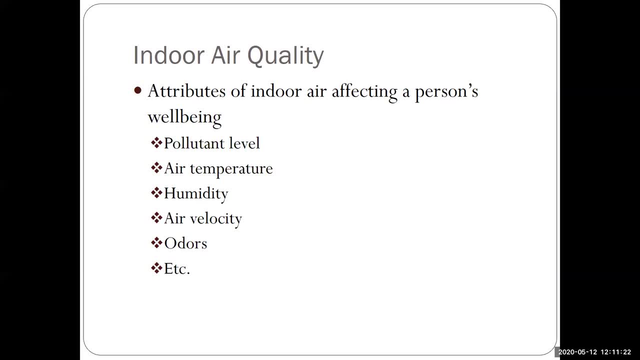 How quickly are we moving the air in and out of a room? And, of course, odors And, as you can imagine, teaching high school students that are working with animals on the farm because, remember, this is an agricultural high school. They've got livestock. 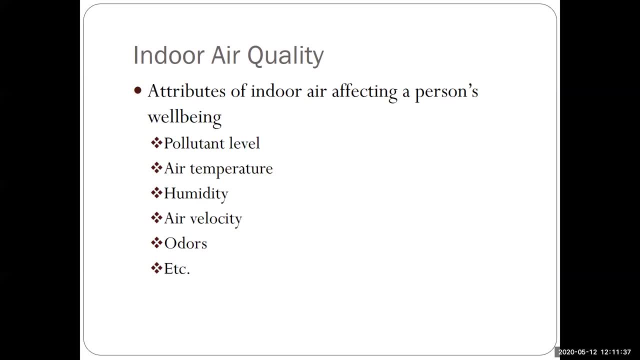 They also have a veterinarian tech program, so they have dogs and cats and other domestic pets. It's just, it's going to smell, And so all of these different things, combined with those traditional pollutants that we think about like gases and particulate matter, 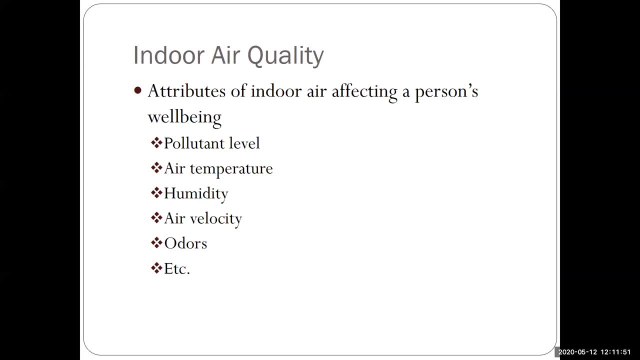 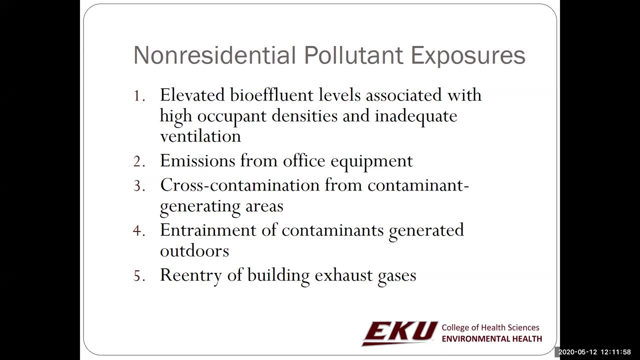 can affect a person's wellbeing if the indoor air quality is poor. I want to go through nine different non-residential pollutant exposures that we have to be mindful of. Number one is elevated bioeffluent levels associated with those high occupant densities and the inadequate ventilation. 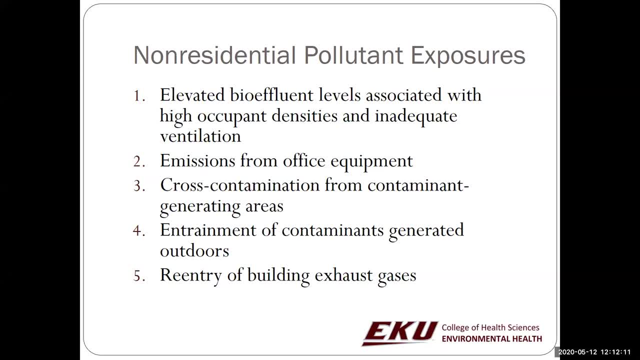 So bioeffluent we mean pollutants that are released by humans and other organisms. We have emissions from office equipment, So things that we have to use to be more efficient in our job can actually cause us to have IQ issues- Cross-contamination from contaminant generating areas. 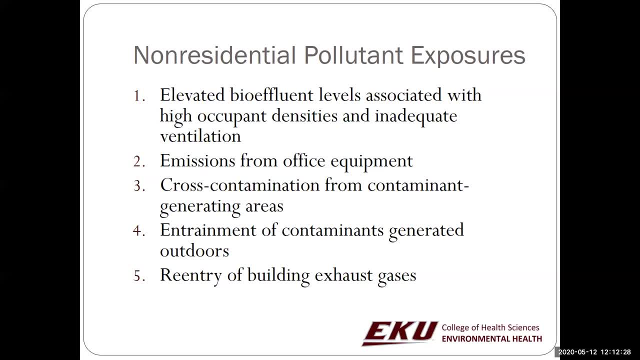 So sometimes we have an area we think it's well ventilated, we have it blocked off or it shouldn't be an issue to other portions of a non-residential building, but for some reason we're able to cross contaminate Entrainments of contaminants. 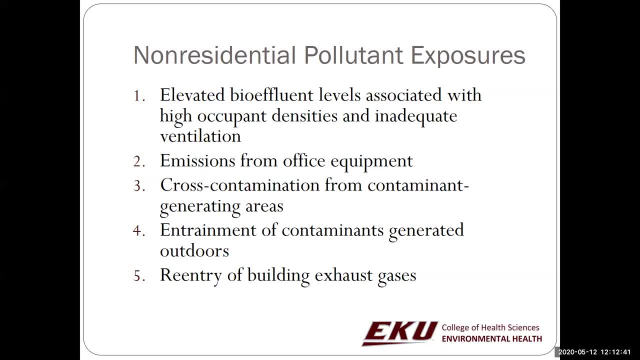 that are generated outdoors. So, opening and closing doors, we pull in air from outside and that can actually bring outdoor pollutants in, creating an additional indoor air quality issue. We also have re-entry of building exhaust gases, So imagine that something is going wrong. 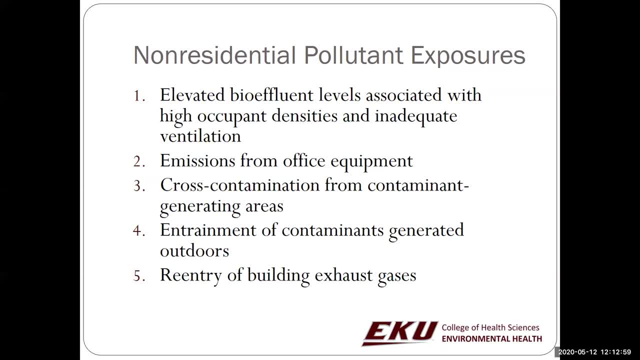 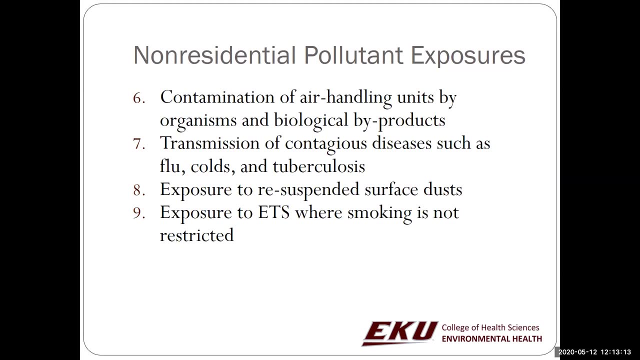 with your exhaust and you're actually pulling that gas back in through your intake and it's being basically circulated through your building. Number two: contamination of air handling units by organisms and biological byproducts, And so you can think of, like legionnaires, disease. 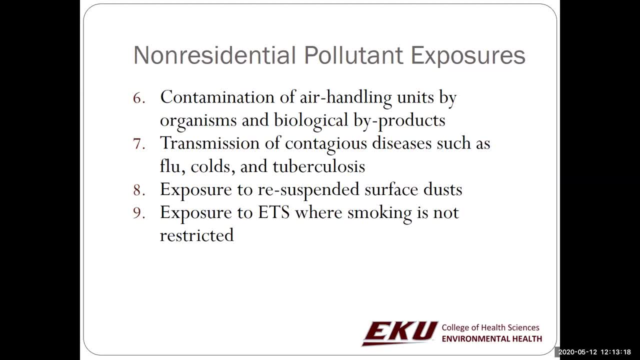 for example. that would be a great example of an air handling unit having a problem and folks are wondering what is going on, and something that should again help us. the air handling unit getting us the air exchange ends up hurting us. Transmission of contagious diseases. 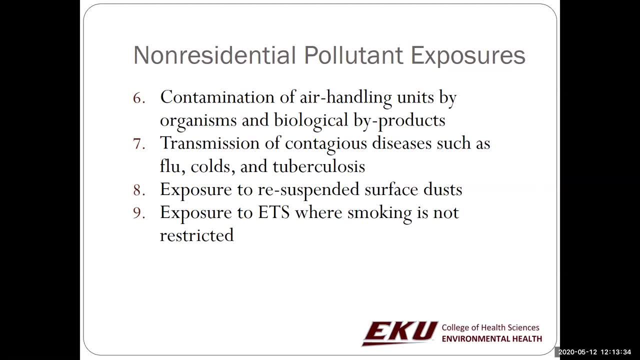 such as flu, colds and tuberculosis, especially flu and colds when you think of the US. these are easily transmitted amongst these folks that are spending a good period of their day together Exposure to resuspended surface dust. So imagine, for example, 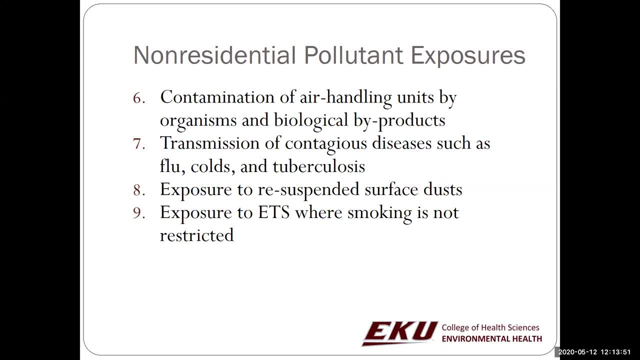 you go in to sweep a room, you kick up the dust. that dust goes back into the air. you now have particulate matter that you could inhale, And then, of course, exposure to ETS where smoking is not restricted, So in a school. 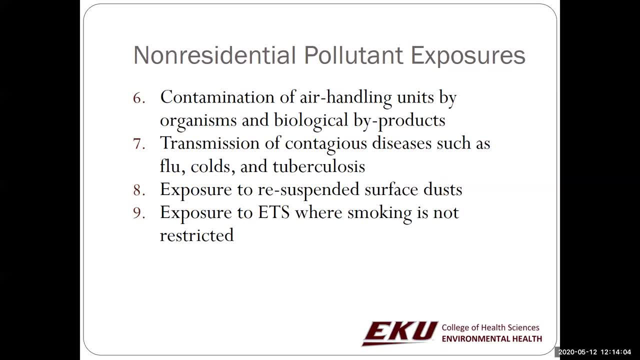 we're not gonna have that issue. So environmental tobacco smoke would not be an issue. but if you imagine a school had a policy where they could smoke- teachers could smoke somewhere on the premises- that could be an issue where it gets pulled back into the building. 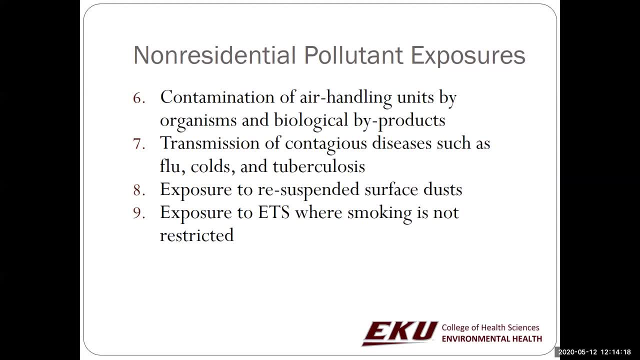 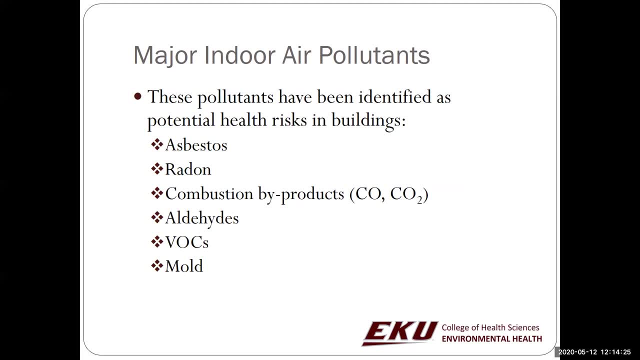 For this particular school it's not because the county had a ban on public smoking. So other issues, major indoor air pollutants that we'd have to be mindful of. asbestos, of course, in older buildings we know it was used for fireproofing. 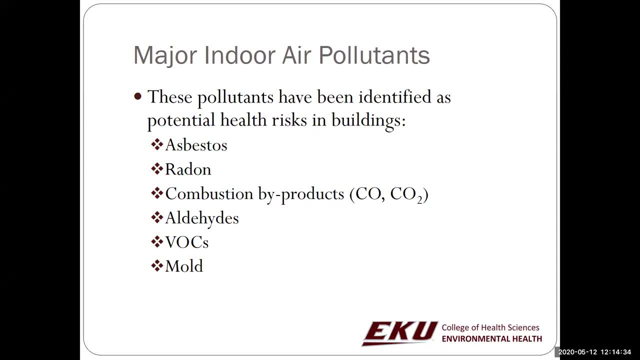 acoustical plaster thermal system installation. We did not have that issue with this particular building because it was built in 2011.. Radon: this is an issue because of where it's located and the topography and the different soil structure underneath the school. 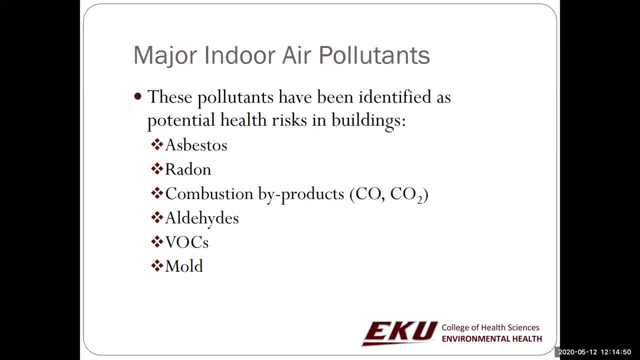 This region is known for high levels of radon, But remember, we have a radon detection system that's built into the school Combustion byproducts, CO and CO2.. So this particular school, as I mentioned, they actually do diesel engine repair. 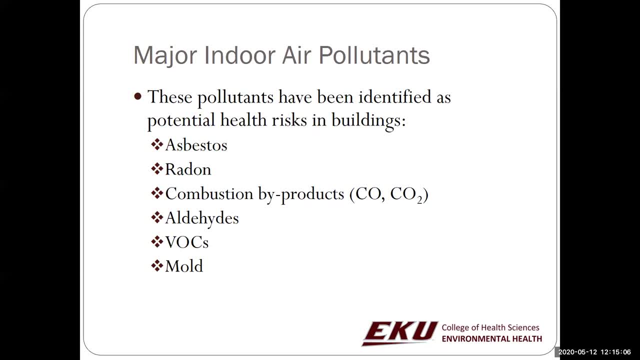 So they work on different forms of different farm equipment that have diesel engines And, as you'll find out through this presentation, the school didn't have the best ventilation system to account for running these diesel engines indoors. Aldehydes, especially formaldehyde. 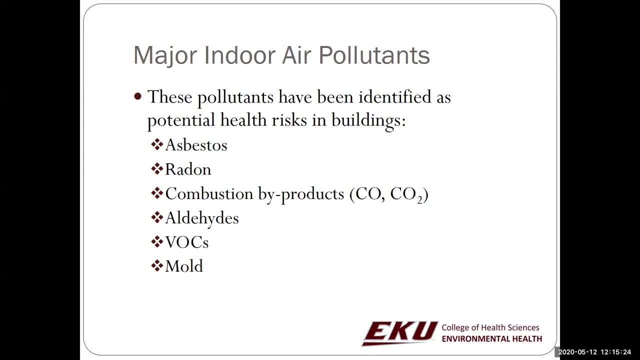 So if you think about newer buildings, most likely we're going to have a lot of compressed wood. We're going to have carpet and other materials that are going to have aldehydes in it, especially formaldehyde, because it's widely used in industrial and commercial chemicals. 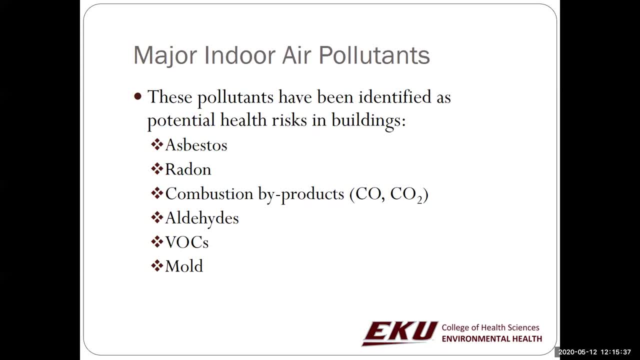 So we'll find it in pressed wood materials, especially particle board, so cabinetry and furniture. If you got it for a good deal, there's a good chance you're going to see the off-gassing of these formaldehydes. We also have VOCs. 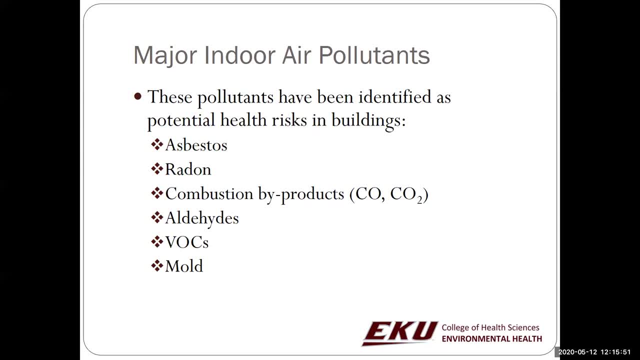 VOCs are going to be common in this type of school because of the diesel engines and some of the other agricultural processes that they have. So volatile organic compounds. they can be emitted from a lot of different sources, But again for this one. 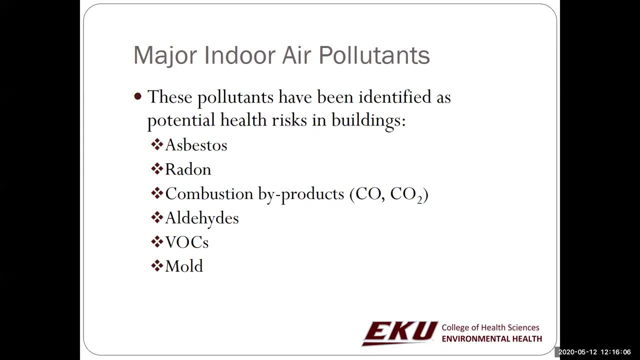 it's going to be from the equipment that they're using. All right, And, of course, mold. Any place where you can have some moisture going on in the perfect conditions, those microorganisms will grow and grow and grow as long as they have. 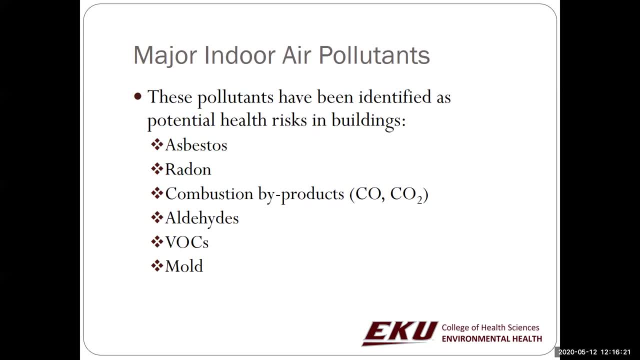 all of the perfect conditions, all the pieces of the puzzle to help them thrive. And in Kentucky, if you're not familiar, Kentucky has a huge mold problem. So this was something we had to be mindful of as we were thinking through the potential pollutants. 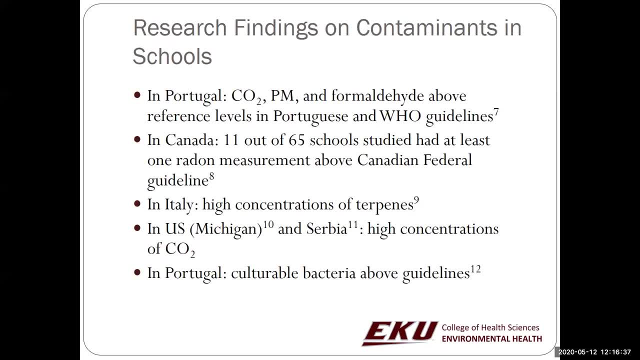 for the school. Now, if you look at the research on contaminants in school, it's all of the usual suspects, But one of the things you'll find is there's not a lot of good studies in the United States. Most of them happen abroad. 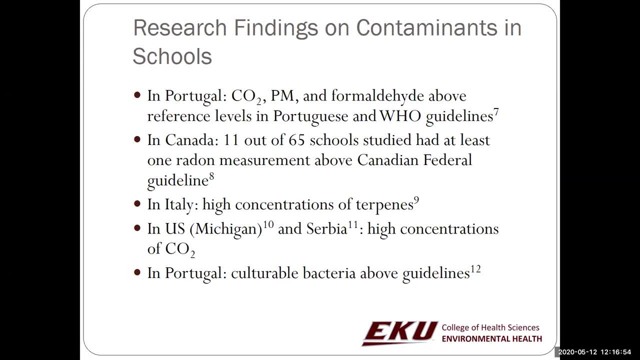 So in Portugal, for example, carbon dioxide, particulate matter and formaldehyde were above reference levels in these Portuguese schools, and they exceeded the World Health Organization's guidelines In Canada. if you read certain literature, you'll see that this particular study 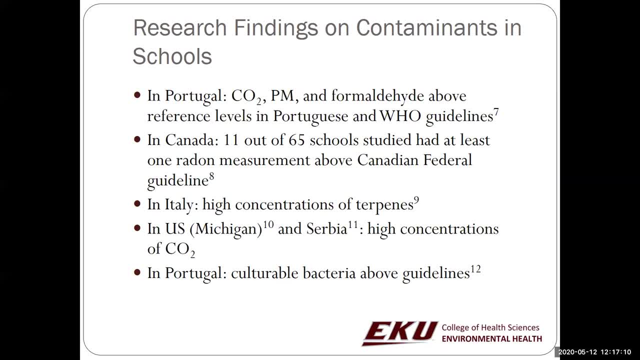 11 out of 65 schools that they studied had at least one radon measurement above Canadian federal guidelines In Italy. we've seen high concentrations of terpenes In the US and also in Serbia, as we would expect with a high density occupancy. 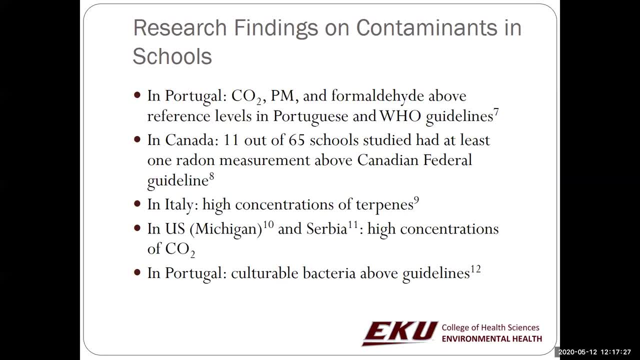 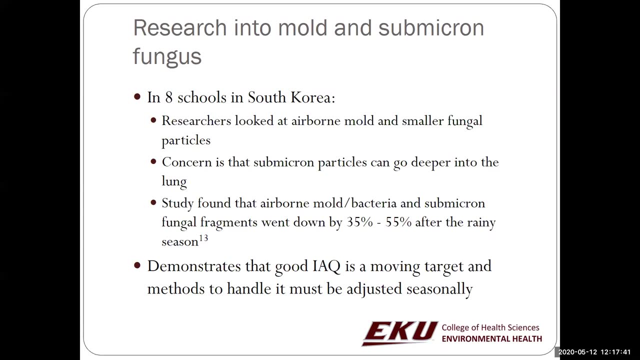 type situation, we had high concentrations of CO2.. Also in Portugal, in a different study, we saw carbon dioxide as a cultivable bacteria above guidelines. So these findings are not surprising, given what we know about indoor quality issues. In a study where eight schools 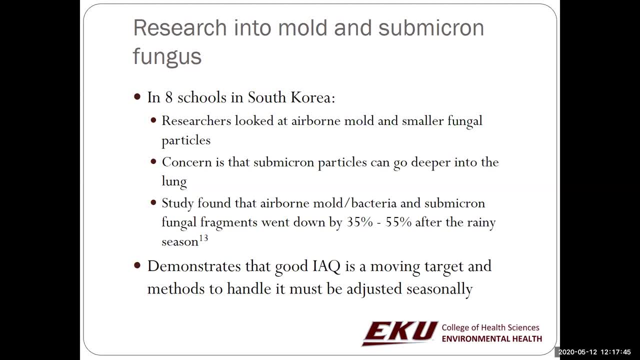 were examined in South Korea. researchers looked at airborne mold and smaller fungal particles and their concern is that that submicron particle can go deeper into the lung, which is something that we commonly accept. The study found that airborne mold and bacteria and submicron fungal fragments 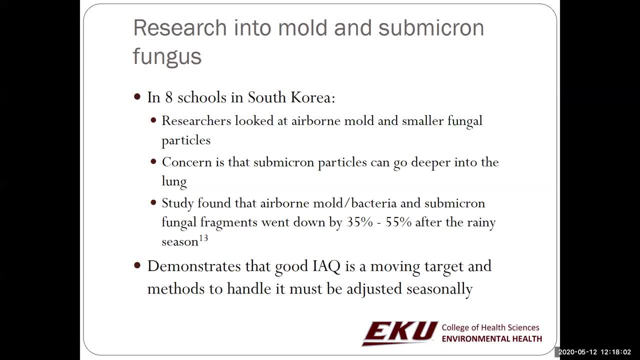 actually went down by 35 to 55% after the rainy season. Okay, this is not earth-shattering news. It's kind of like Kentucky: We know what time of year we're going to see higher fungal growth, right? We just so happen to be doing our study in January. 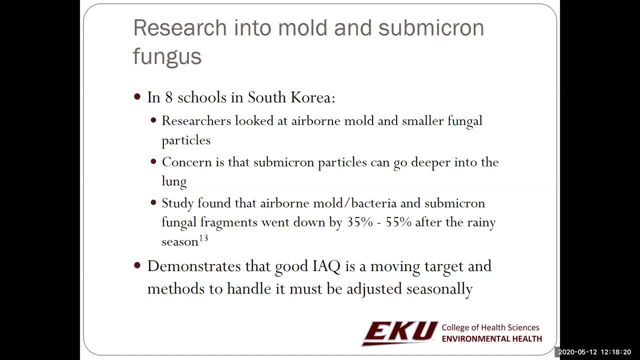 So it's very cold. in Kentucky We get a little snow, Temperatures are in the 30s and 40s, So we don't see as much issue with the fungal growth. but we do see a lot of issue with folks passing on colds and influenza. 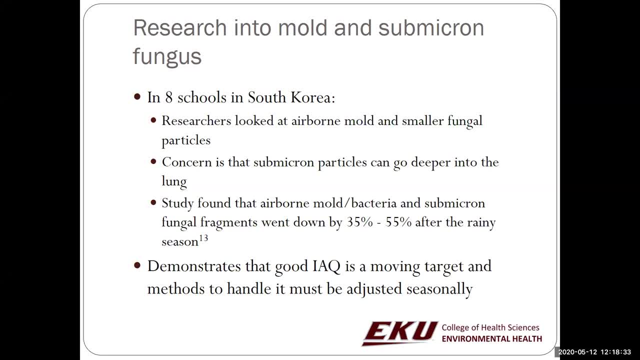 So what do we take away from this particular study? It tells us that good IAQ is a moving target and the methods to handle it must be adjusted seasonally. So we have to control, for the season, the temperature. what's going on with the weather? 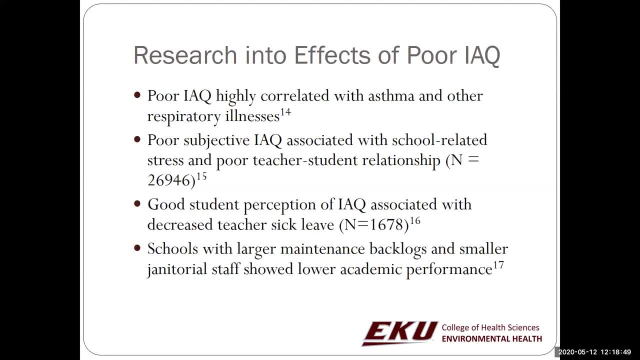 when we start looking at the potential IAQ issues. A few more studies before we move on to this particular study in the Midwestern portion of the United States, Poor indoor air quality is highly correlated with asthma and other respiratory illnesses. Again, not earth-shattering. 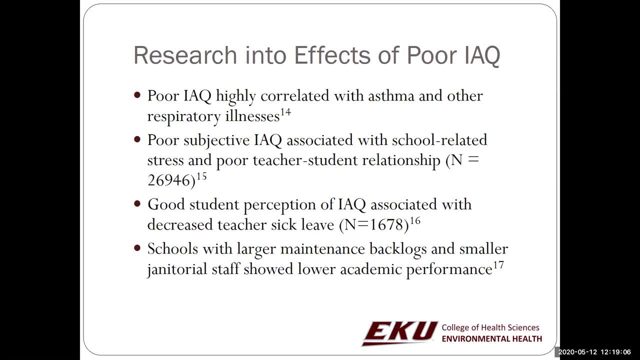 but it's something we have to point out because we have a lot of students that are going to be suffering from asthma and other respiratory illnesses, So they're more susceptible to these indoor air quality issues. Poor subjective IAQ is associated with school-related stress. 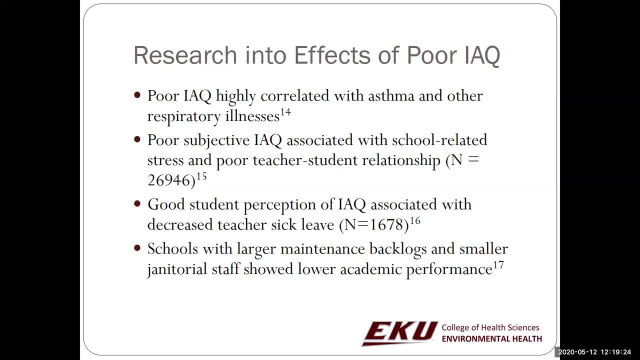 and poor teacher-student relationship. So basically, what we're seeing here is, if the IAQ goes down, even in perception, we're going to see more strain between the teachers and students, which is going to impact the ability of the teacher to instruct. 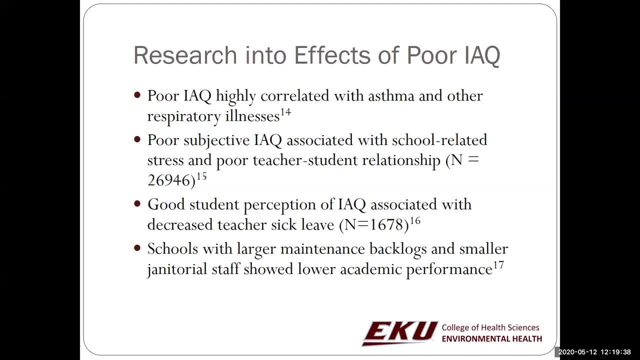 at his or her optimal level. but it's also going to impact the student's ability to take in that information and learn. Good student perception of IAQ is associated with decreased teacher sick leave. So when students found the indoor air quality to be agreeable to them, 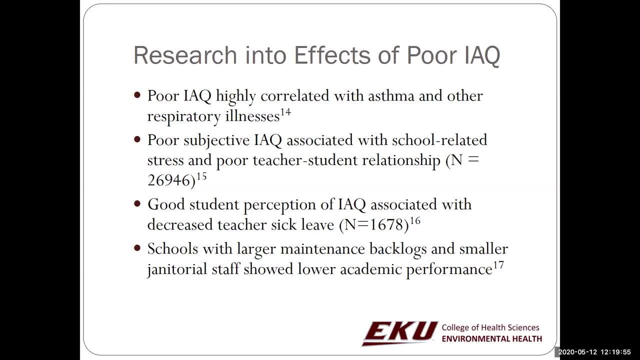 we noticed in literature that teachers were less likely to miss. They were more likely to be there to be engaged and to be instructing. Another thing that's interesting is schools with larger maintenance backlogs and smaller janitorial staff usually show lower academic performance. 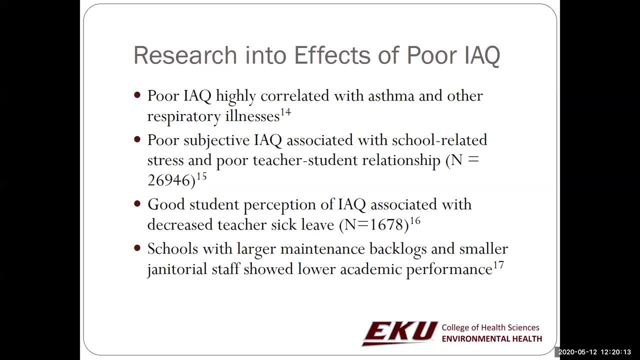 This is something to think about in a very budget-oriented world that we live in. Sometimes school administrators think of the maintenance budget as soft money that they can get rid of it without really affecting their academic performance. However, the negative health effects for students and teachers. 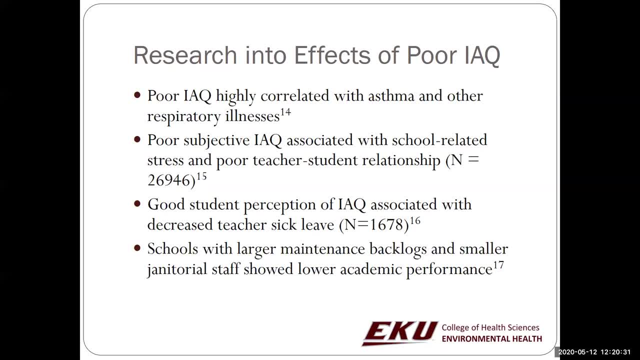 demonstrate that you must maintain good indoor air quality. It's core to the academic success of the school and it's also core in building those relationships between teachers and their students. So that's a little background. We talked about a few indoor air quality pollutants. 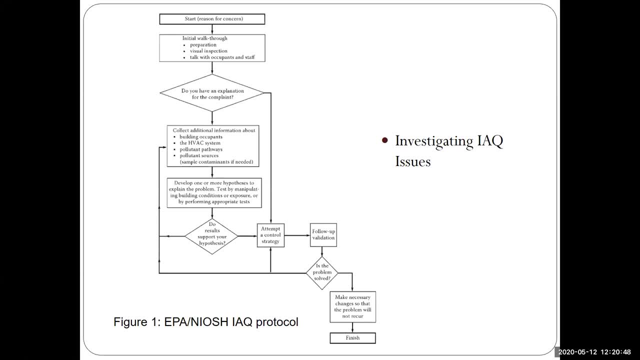 We looked at some of the literature. So now we're going to go through what my colleague and I did for our particular case. Recall that we're dealing with an agricultural school. It's a net zero energy facility. It's a magnet school. 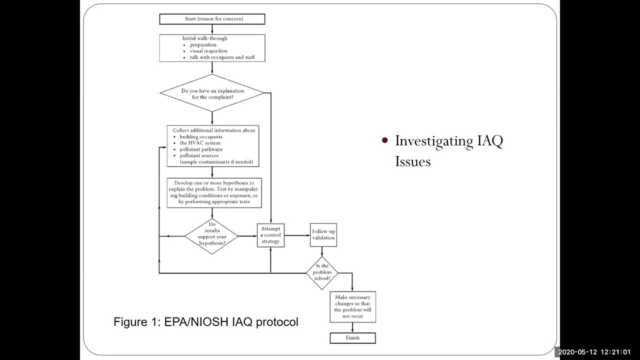 so the students aren't there all day, but the teachers are. So we decided, of course, to use the EPA, NIOSH, IAQ protocol. It's standard. I think it's marvelous because it keeps it straightforward and you can kind of work yourself. 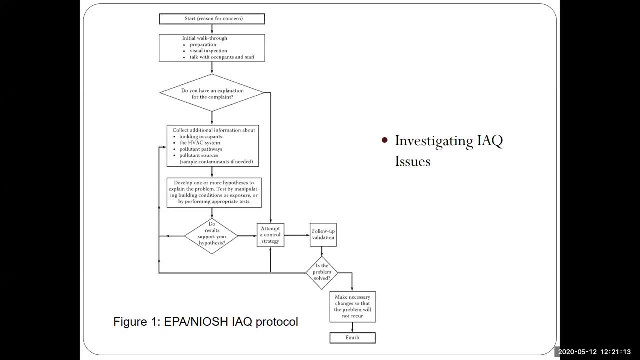 back through it when you think you have the answer but the data aren't supporting it. So if you look at this figure, figure one, you start with your reason for concern. So our reason for concern was that the teachers were complaining about headaches. 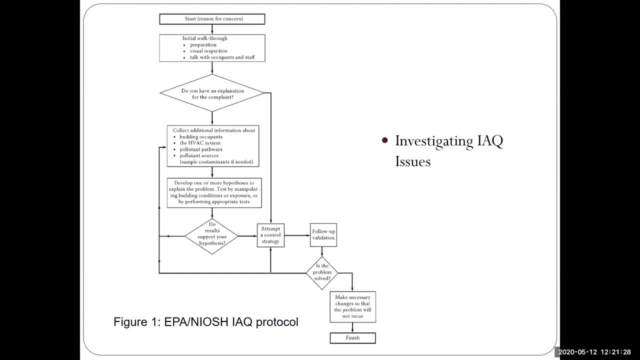 coughing kind of cold symptoms could be allergy symptoms and they had gone through several IAQs in the past. Several IAQ studies have been conducted. The industrial hatchetist would come back and say there's not an issue. 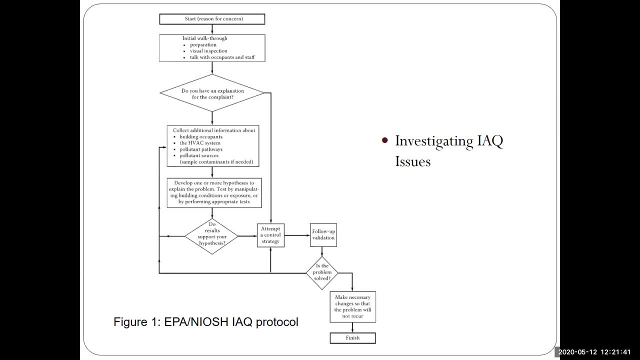 Everything's coming back under the appropriate parameters. So what we did was we started off with a meeting with all the faculty, the staff and the principal of the school. We wanted to tell them what we were about to do in the school. Full disclosure. 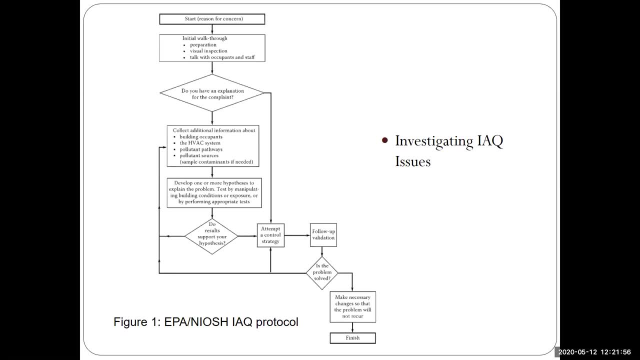 we wanted to be transparent. We wanted to get that buy-in from them, from the get-go, which is very important. We all know that's like management 101, right Stakeholder buy-in. So we go to the school, We tell them what we're going to do. 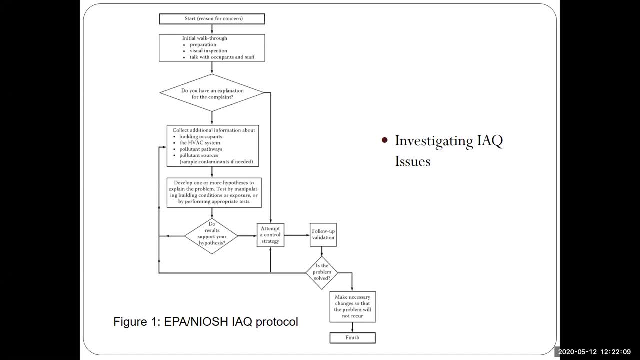 We tell them the type of instruments we're going to use, our timeframe. We give them our contact information so that if they do have questions, that they could follow up with us. We also tell them that during our IAQ study we were going to encourage them. 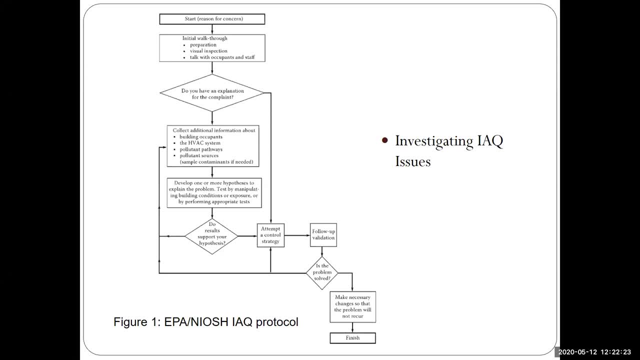 to complete a self-perception questionnaire. It's an indoor environmental quality survey where they get to tell us what type of symptoms they're experiencing. Do those symptoms get better when they leave school? They get to tell us about their workday, their workstations. 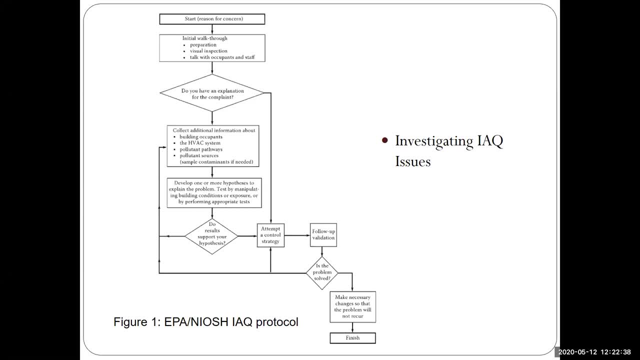 And then there's also just some open response questions where they can tell us any type of information they think is pertinent to the study. So we give them this information. Everyone seems good to roll, And so we then go through and do our initial walkthrough. 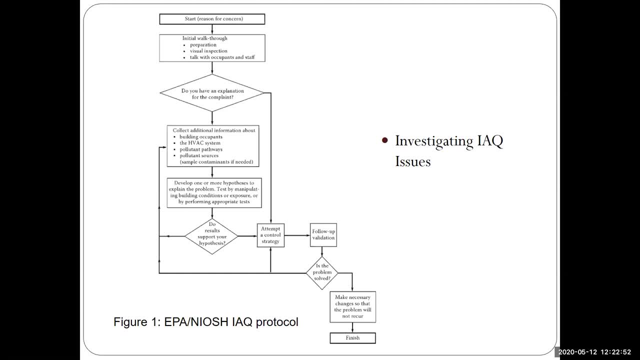 So for us, we identified where the HVAC intakes and outlets were. We figured out all the major classrooms of the teachers that were having the biggest issues with symptoms. We looked basically throughout the school for fungal growth. We looked throughout the school for any issue that could be causing. 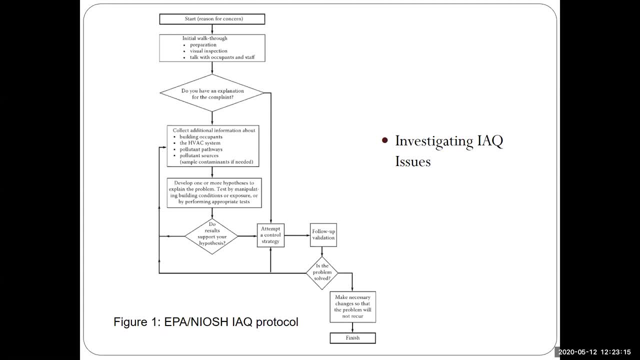 indoor air quality problems. So we do our visual inspection. We also do some interviews with the occupants. So we do interviews with the teachers and we do interviews with the staff. We do interviews with the front office staff, the principal, And so then we start thinking through. 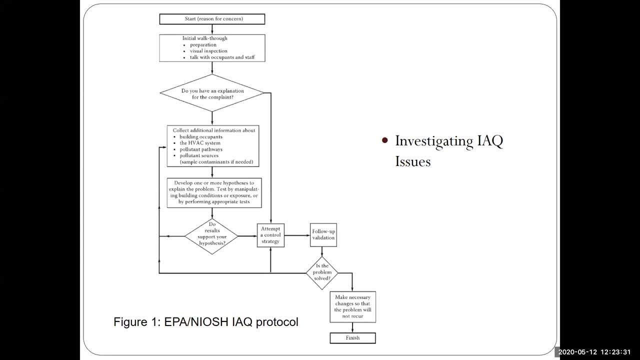 obviously do. we have any explanation for the complaint, And so for us we had to align that also with doing some monitoring. So we're going to go back to this particular figure later in the presentation. I just wanted to get you started out. 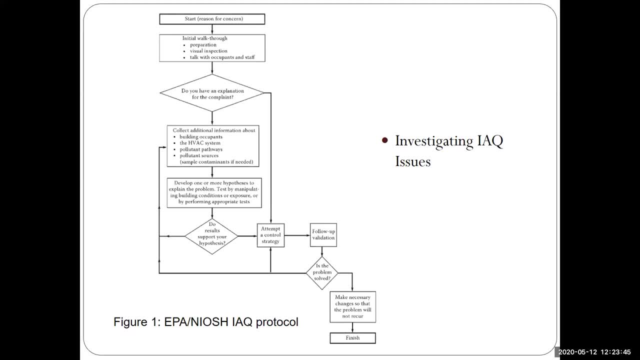 where we were at. So our hypothesis basically was that, based on what they were telling us, we probably had high CO2 levels. but of course we had to do monitoring. We wanted to make sure that we had additional information on the potential pollutant sources. 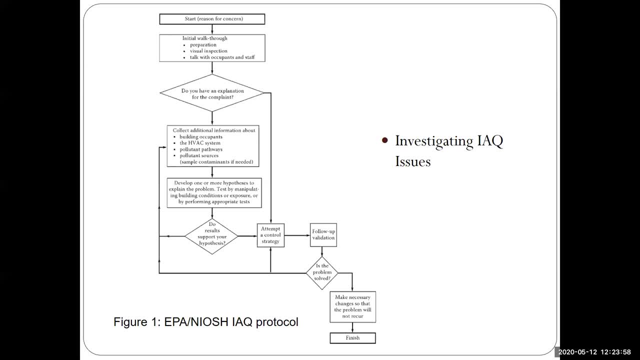 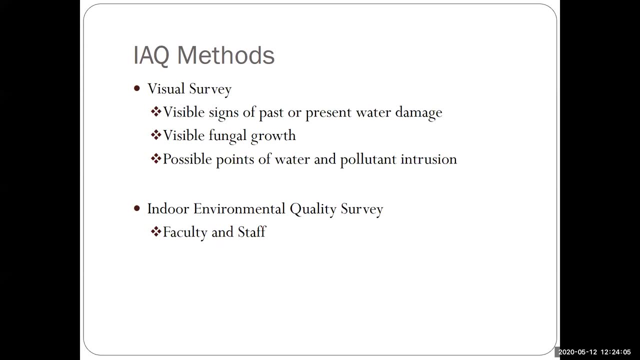 the pathways from the source to the inhabitants. All right. So our methodology: we did the visual survey. So, of course, like I said, we did a look for visible signs of past or present water damage. We looked for visible fungal growth and we looked for possible points. 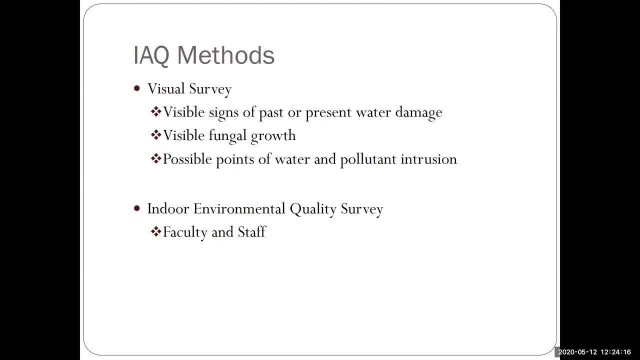 of water and pollutant intrusion Right. And of course we left the survey in the boxes of all the faculty and staff in the front office For them to pick up and then drop off in the library. We wanted to do the library because we felt like that gave. 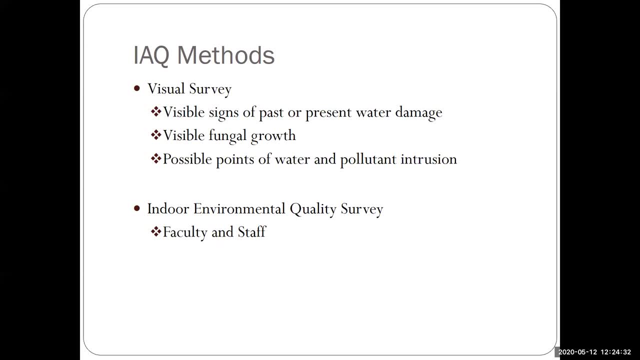 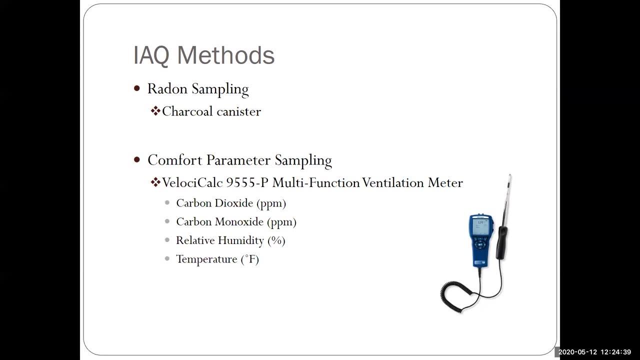 the faculty a little more control over who saw them, you know, turning in their survey, just in case, only a few people completed it. We did do radon sampling because the school had a built-in radon system And, of course, this particular area of the country. 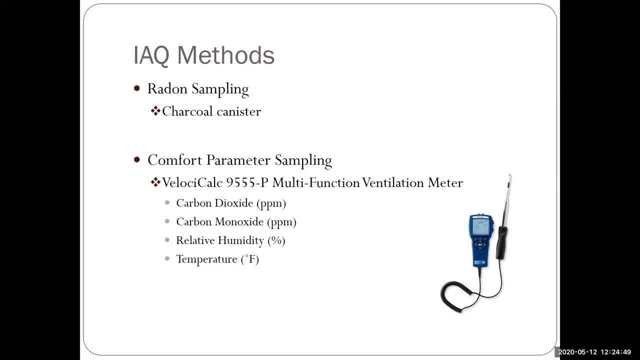 has issues with radon. We wanted to go ahead and do a charcoal canister sampling. We built our plan. We based it off of pretty standard EPA school guidelines for assessing radon. We also did comfort parameter sampling, So we used several Velocicalcs. 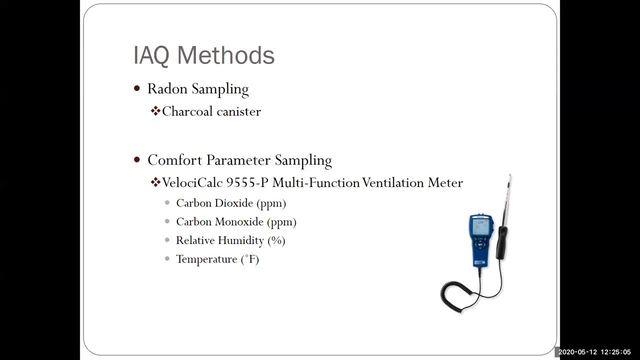 the 955P multifunction ventilation meter And, if you're familiar with it, the Velocicalc is capable of reading carbon dioxide and PPM, or parts per million carbon monoxide and parts per million relative humidity in percent and then temperature in degrees Fahrenheit. 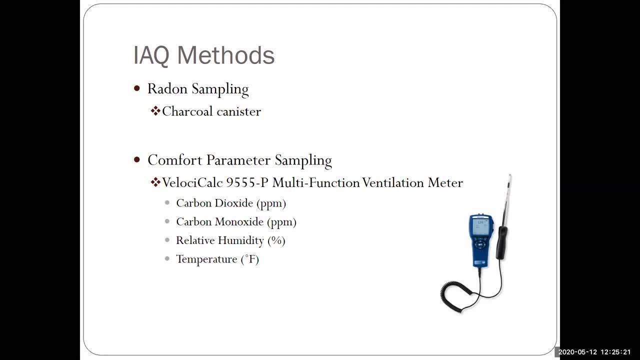 So we had five of these that were set up throughout the school And what we would do is rotate them by day so that we would ensure we got the hallway, we got classrooms, labs, offices- a full study of the school in terms of these comfort parameters. 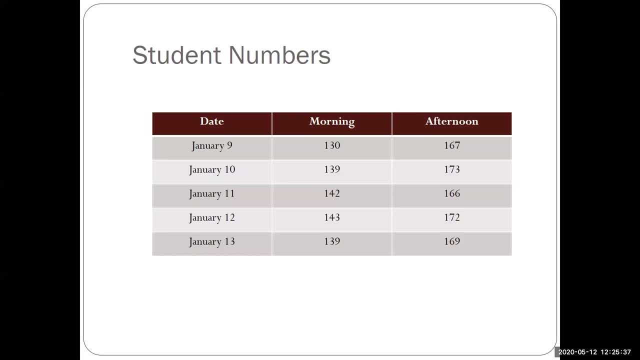 As I mentioned, students don't stay all day at the school, So this is just kind of a breakdown on the days we did it- Remember it was in January. We had roughly between 130 to 143 students at any given time in the morning. 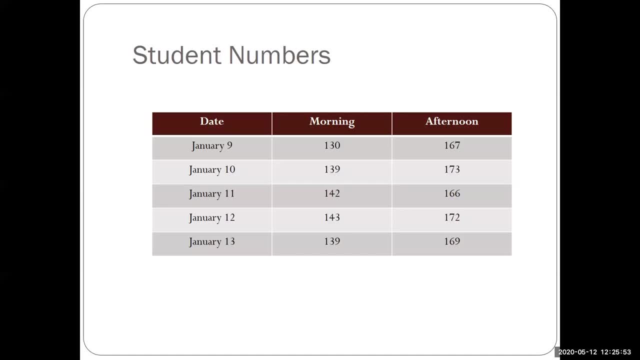 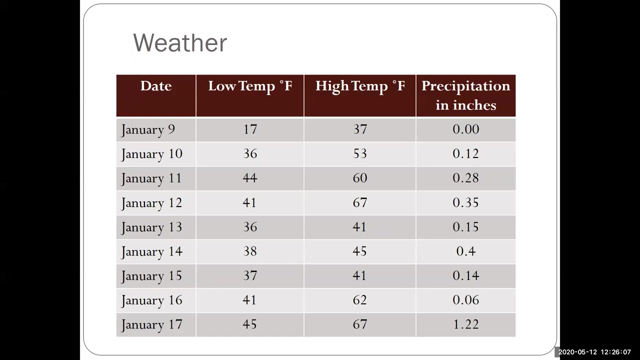 in the classrooms, And in the afternoon the number grew a little between 166 and 173. So it wasn't a huge student population, but they tended to be in certain classrooms at particular times during the day. This was the weather during our studies. 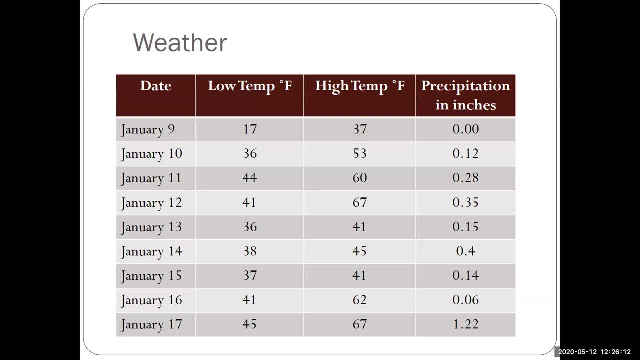 So we did the IAQ comfort parameter testing the 9th through the 13th, And then we also did the radon for an extended period of time over the weekend, while they were shut down in observance of Martin Luther King Jr Day. 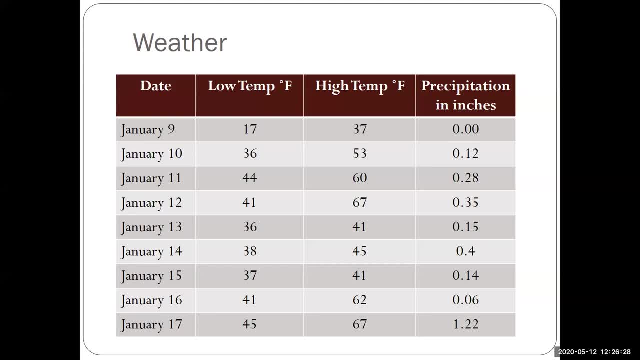 And you can just see this, the temperature range. it started out pretty bitterly cold, but then by the end of our study it was getting higher during the day, which is a typical Kentucky weather day. If you don't like it, just give it a couple hours. 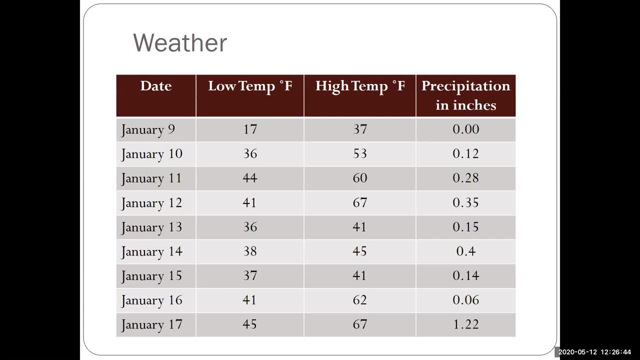 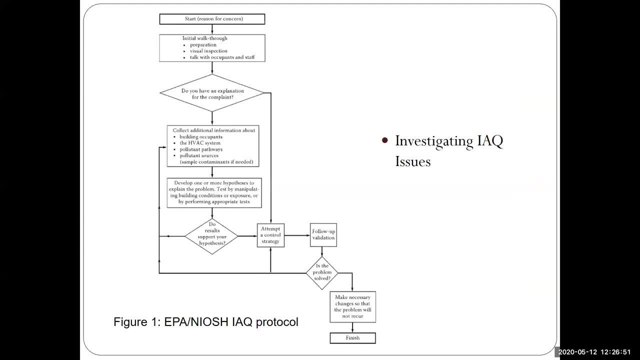 It'll change, I promise, And you can see the precipitation there. So towards the end of the study, we did have more precipitation that was falling in the area. So, coming back to this, we do our study. I want to give you some of the data. 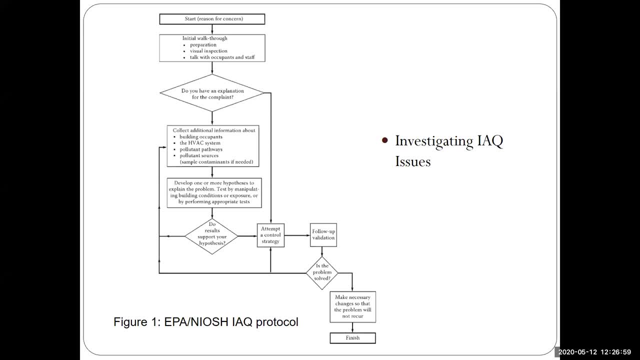 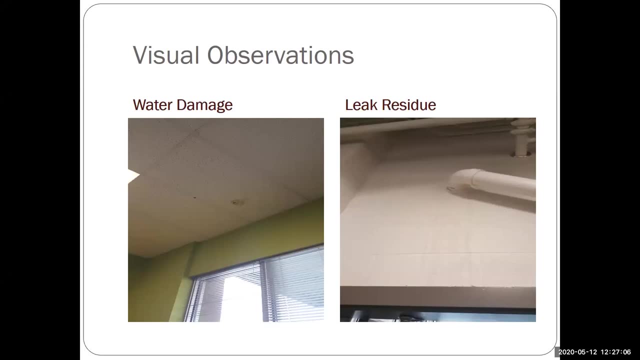 that we were using to either support or go against our hypothesis. So some of the visual observations that we made. So, as we were walking through, we noticed in several places throughout the school water damaged tile. Now this does not necessarily mean that we're gonna have fungal growth. 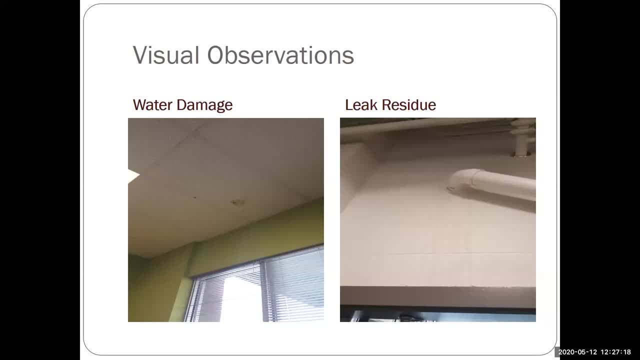 but it does tell us that we have a water source that's uncontrolled, which could lead to fungal growth. This one just so happened to be in the front office of the school On the right. you'll see that we have leak residue. 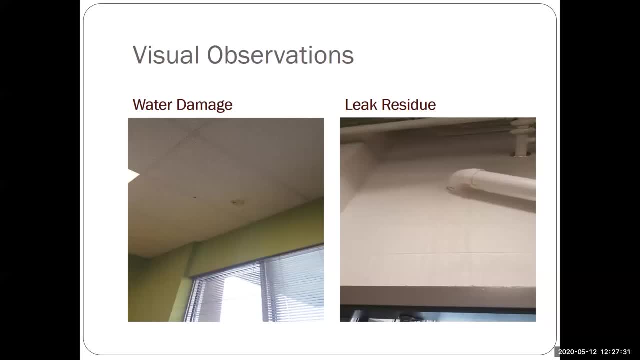 So something was coming from this pipe. We talked to maintenance. They weren't really sure what was going on, but this again told us that something is off here. Things are not being controlled. Maybe they could do a better job with their maintenance plan. 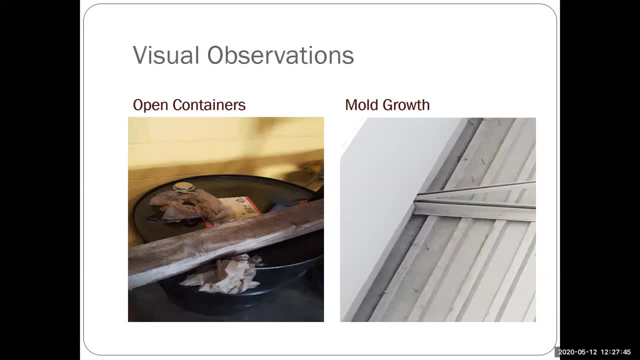 Some of my favorite pictures. If you look at the one on the left here we see in the diesel mechanics, there's a pretty good example of what this might have done. This is just a drop in the first one on the left, This is a picture of how that might have worked. 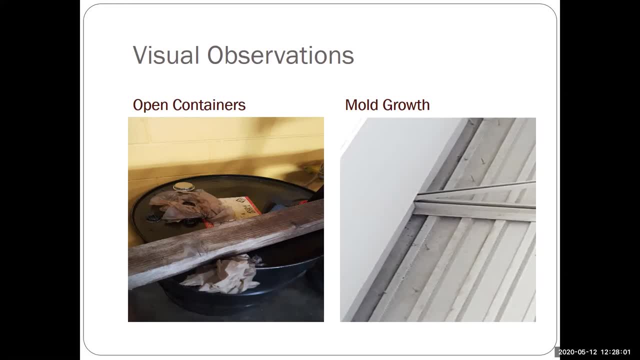 if we were out at the teacher's desk. But we definitely found that while theeman was working on the project, the teacher was giving the students a lot of examples of how this could be a problem. So we found that this was a problem. The teacher involved in the construction. 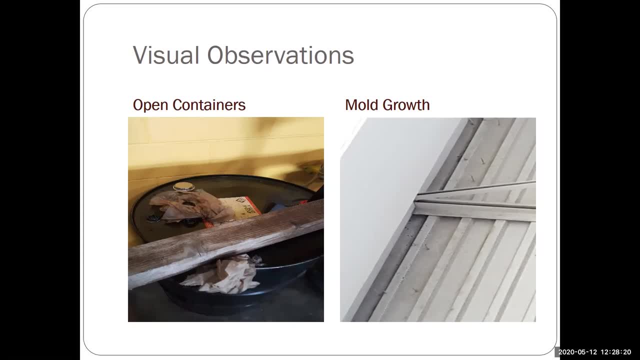 of the location of the whole building. We just saw some sort of discoloration. It was very high off the ground. It was part of a follow-up study that we weren't contacted to do. Okay, on the left you'll see that there's some repair. 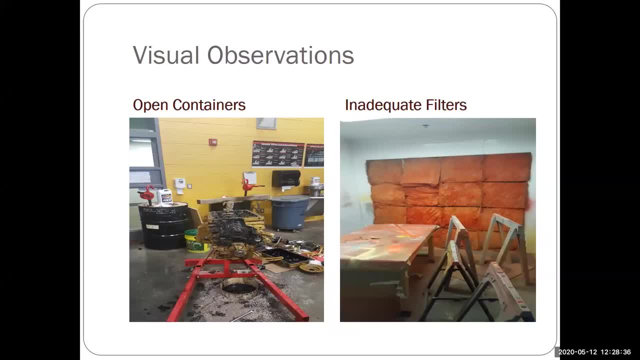 happening to an engine. This was being done in a room that was not designed for this type of mechanical work. It was actually designed for horses because, remember, this is an agricultural school and so they had an equine program, They had a veterinary tech program, so this particular 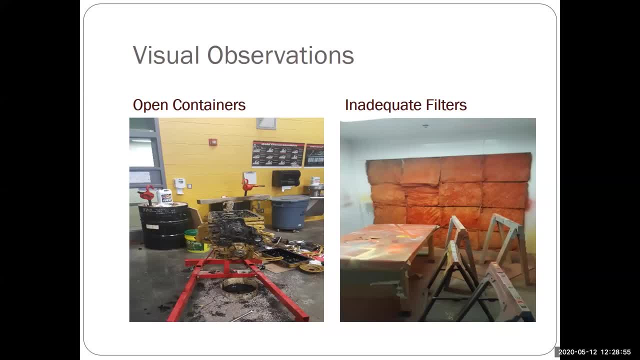 room was built for horses, and they had just basically turned it into a diesel mechanics room, but didn't change the ventilation, and so if you look on the right, you see a paint booth that clearly needs filter changing. Students were observed conducting grinding on a table outside. 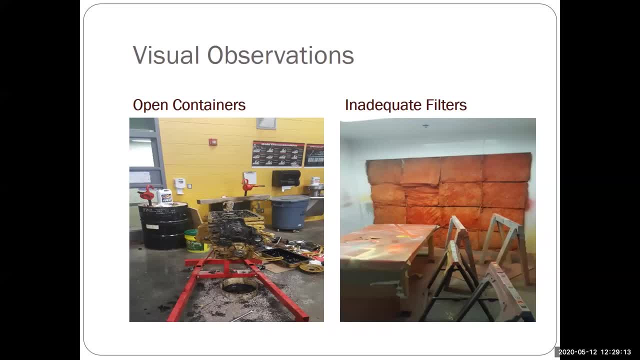 of the paint booth. The paint booth was being used as the ventilation which, as we all know, provided minimal to no protection from the air. The paint booth was also poorly located for a lot of the activities that took place in the laboratory, so many of the things they needed to paint could not get into the actual paint booth. 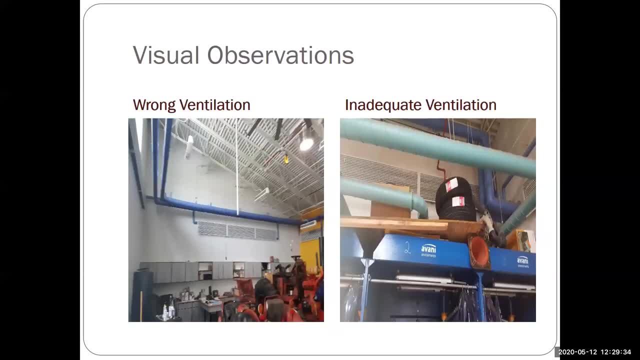 which caused them to paint them in places that didn't provide adequate ventilation. Here you can see they've brought in some tractors. on the left, The ventilation is actually dropped down from the ceiling, but that again was for horses, so it was not at the appropriate. 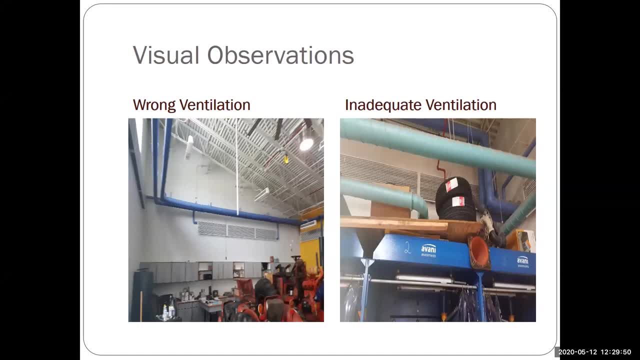 levels for the type of work they were doing. They just had the general ventilation you would have with the classroom, not for diesel mechanics. On the right you can see the ventilation booths that they were using for certain types of welding. When we did just a quick study on the rate, everything was too low. There was no way that it was actually pulling in what it needed to protect those students. Another thing we noticed, which is just like the safety person in me- all these things being stored on top of the paint booth. 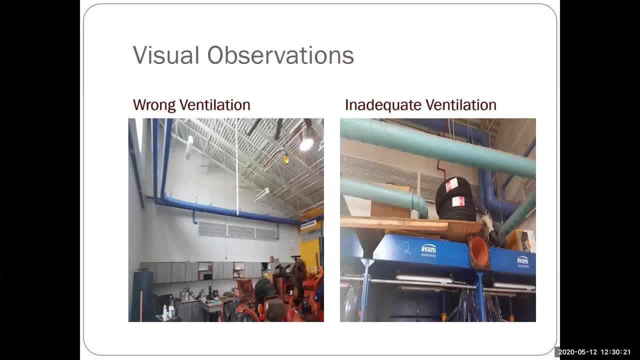 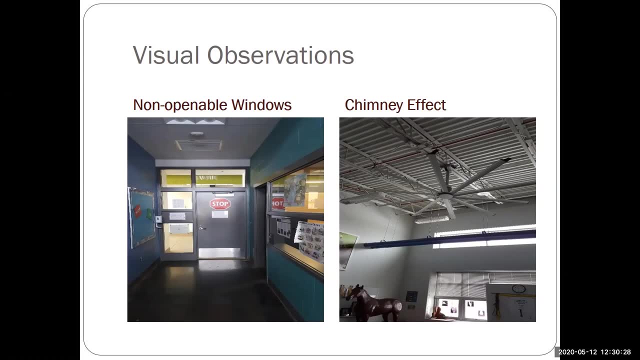 the actual booths, which is a big no-no. Some other visual observations that we saw: The hallway led into each of the classrooms and labs through these little corridors and, as you can see, each of these corridors had windows that could not open. All right, and what was interesting is the hallway itself had no exchange. We could not find any. 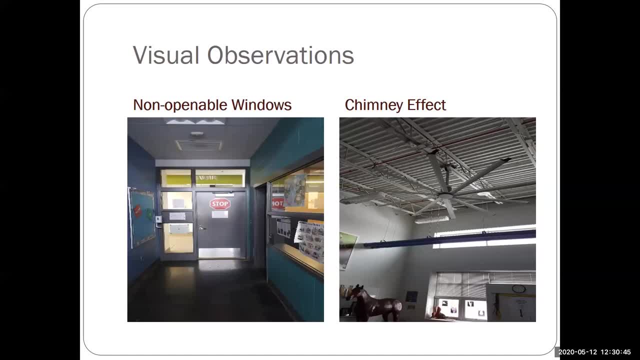 inlets, outlets, anything like that associated with the hallway, and it essentially was supposed to be a temperature-controlled area where they would maintain it at a certain temperature in winter and a certain temperature in summer, and for some reason it would not stay in those parameters while we were there. 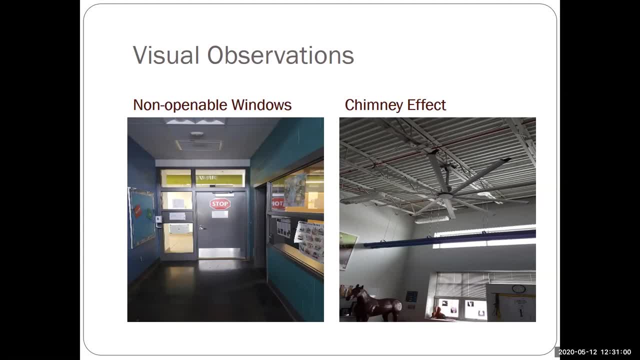 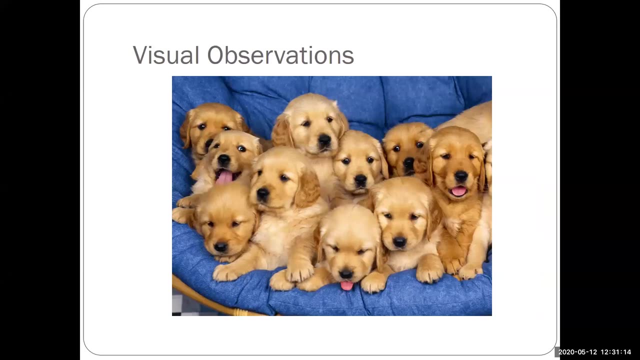 You can see the pitched ceiling on the right. This is where we were seeing some chimney effect, where the warm air would just rise up and kind of get captured there, causing the potential fungal growth. Another visual observation: No, I did not get to experience all these lovely puppies while I was. 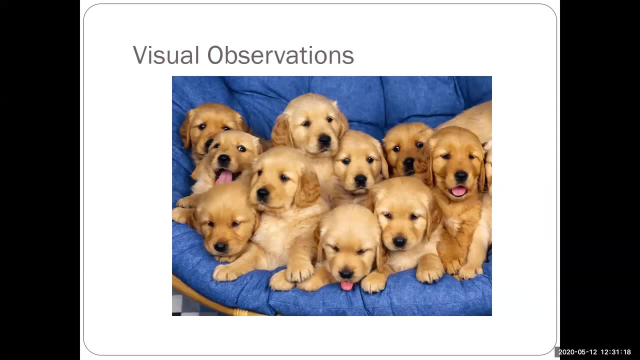 there, but I did see several teachers that were bringing their personal pets to school. Now, mind you, it is a vet tech school in addition to the agricultural piece, So they had a whole section of the building where students were earning their vet tech certification. 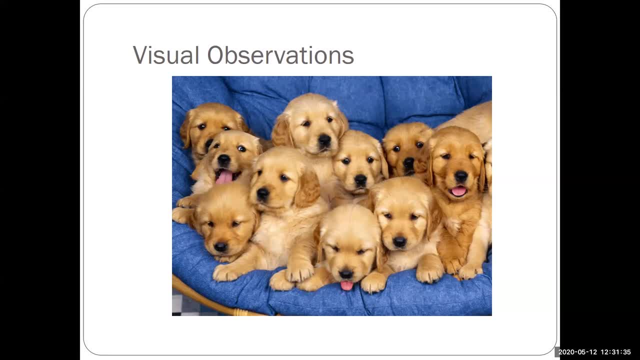 and so it's just natural that you would see animals there. but the animals were brought into the vet tech area through an external door So technically there was some control over where those animals would go in the building, which could minimize some of the biological issues that we would see some of those biofluent. 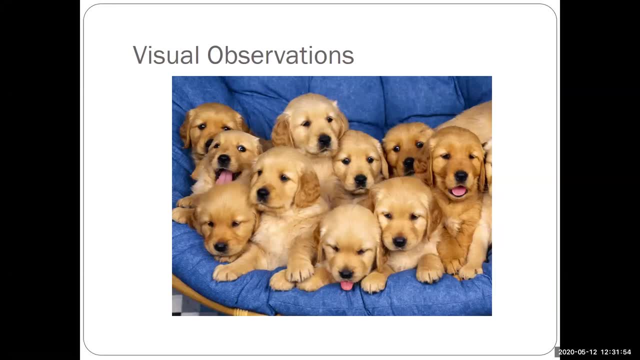 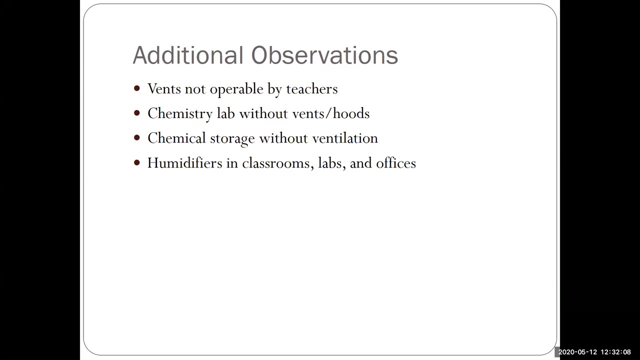 indoor air quality issues. The teachers were taking them to their offices, classroom spaces and just letting them kind of free range. So that was one of the things that we saw as a potential issue. Additional observations that we saw: The vents in the rooms were not operable by the teachers. 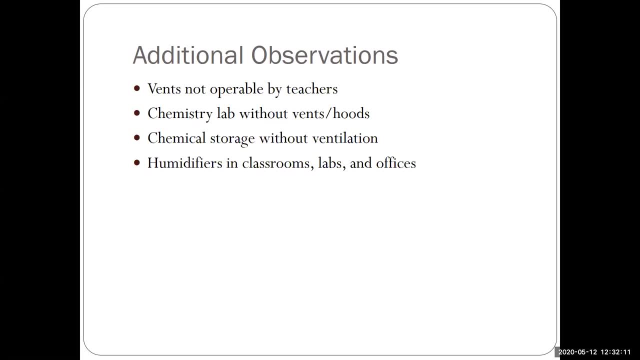 so they really had little to no control over that. We noticed that in the chemistry lab they didn't have vents, They didn't have hoods. They basically were doing chemical reactions in different chemistry laboratory projects without any ventilation other than like your natural exchange you would get in. 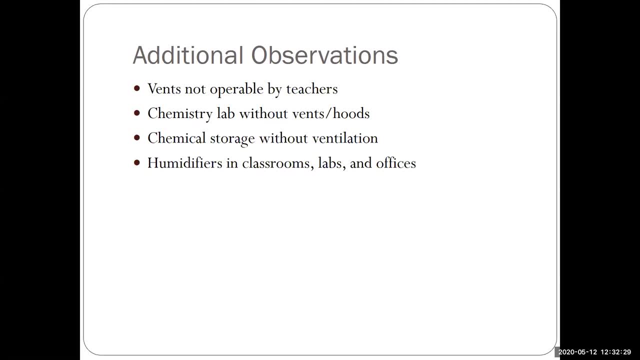 the room. They had a chemical storage room that had zero ventilation, which was a huge red flag for me because, as you can imagine, here you are throwing all these different chemicals and if you didn't put the ventilation in, that tells me that you might not be up. 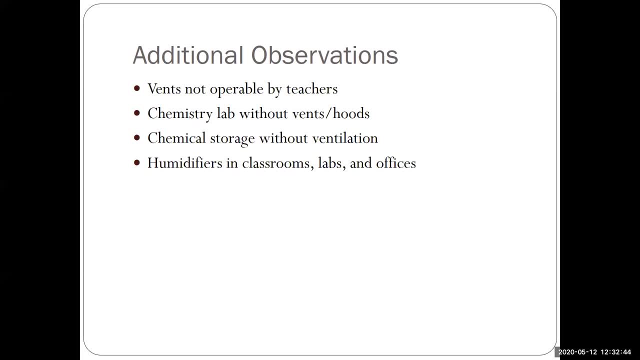 you know, up to par with the type of training you would want to have. And then we had a lot of dehumidifiers in classrooms, labs and offices and what we saw was that the relative humidity was low in a lot of the rooms. 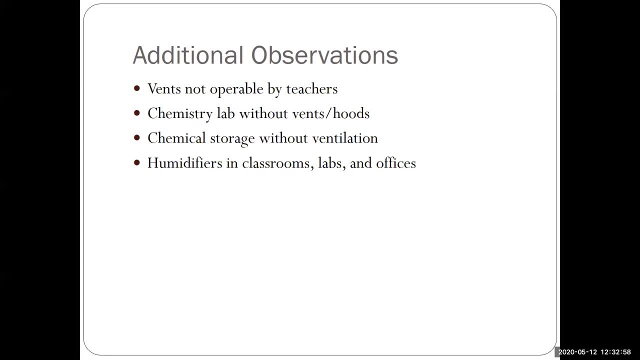 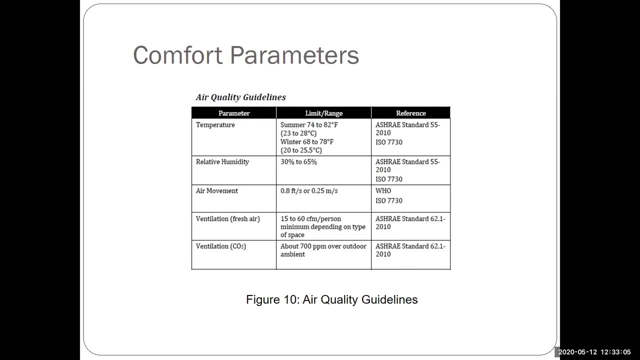 So of course, we would probably would see the itchy eyes, itchy throat associated with lower relative humidity. And so when we're looking at the comfort parameters- remember that's what we use Velocicalc to measure- We were able to measure temperature, relative humidity, and we were also able to obviously 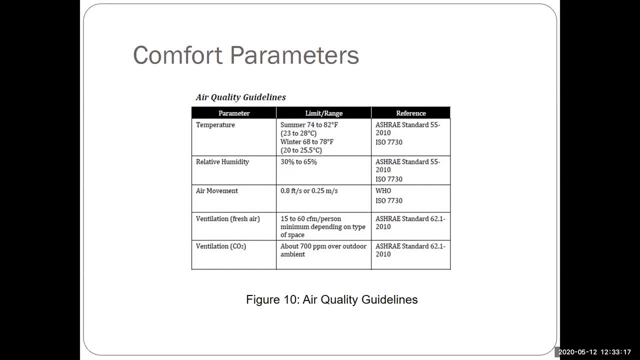 measure CO2 and CO, So this just gives you the standard. So for temperature, for example, where we want to be by the ASHRAE standard 55 from 2010, is between 74 to 82 in the summer and 68 to 78 in the winter, So we were in the middle of winter for Kentucky. 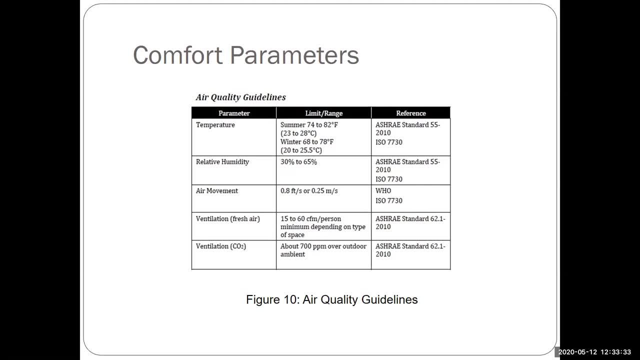 so we should have been between 68 and 78 degrees Fahrenheit. Relative humidity should be between 30 to 65, but if you're on that lower end and you're starting to experience issues, you may want to bump it up a little just to have some humidity in the air. because of the humidity in the air. So if you're in the middle of the winter you may want to bump it up a little just to have some humidity in the air because of the humidity in the air. So if you're in the middle of the winter you may want to bump it up a little just to have some humidity in the air. 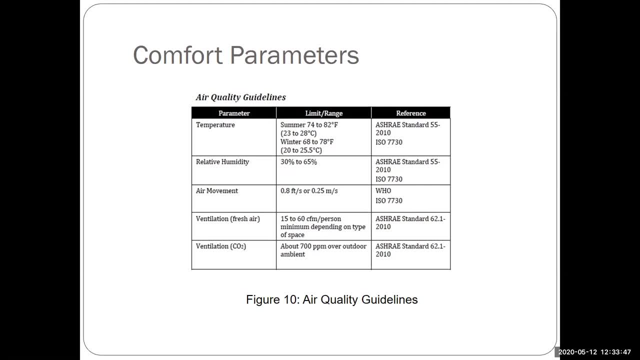 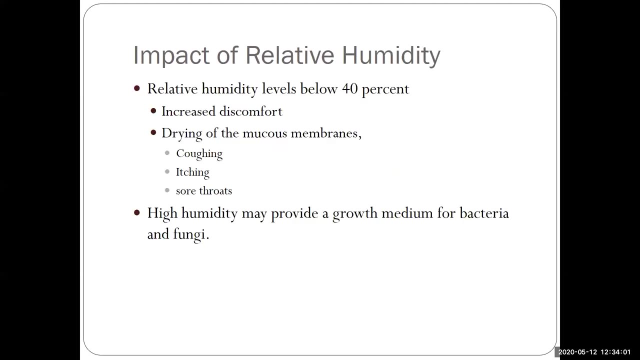 of the dry throats and some of the symptoms we were being told about from the teachers. If you look at the ventilation, looking at CO2, about 700 parts per million over outdoor ambient concentrations is what we would want. So what were we actually finding? We were finding relative. 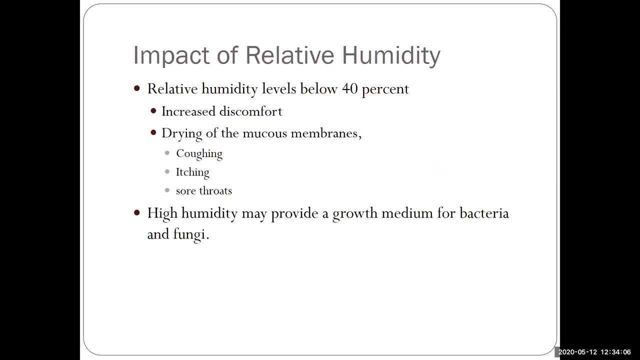 humidity levels that were well below 40 percent. And of course we know when we see that in a school with a lot of folks, a lot of young bodies coming in and out during the day, you're going to have increased discomfort the longer they are in these classrooms And of course, over time you can. 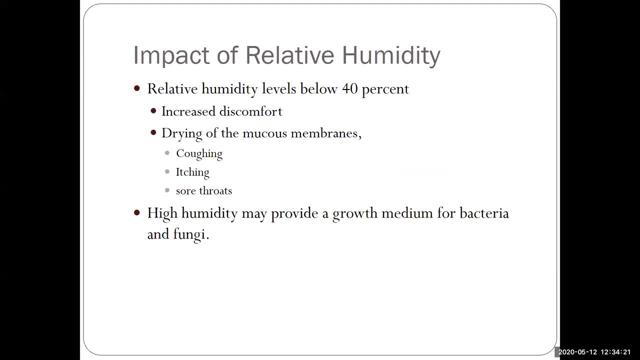 have drying of the mucous membranes, you can have coughing, itching, sore throat and, of course, on the opposite end of that, if we had areas of the building with high humidity, we could see it being a perfect place for bacteria and fungi to grow. So most rooms were below the recommended. 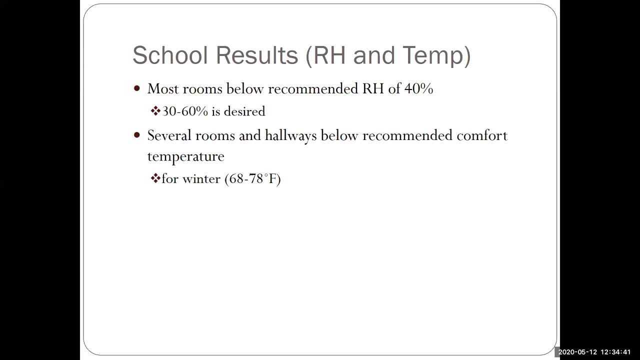 relative humidity of 40 percent. As we said, 30 to 60 is desired. Several rooms and hallways were below the recommended comfort temperatures of 68 to 70 degrees Fahrenheit. Quite frankly, it was very uncomfortable the entire time that I was there and I had on a coat and a toboggan, which in 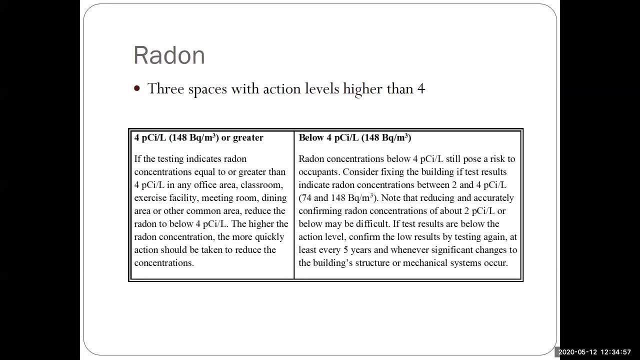 Kentucky means a hat, just in case you don't know. For radon, we did find three spaces that had action levels higher than four, and those spaces were in a caretaker's apartment that was associated with the barn. All right, so again, four picocuries per liter, that's going to be our action. 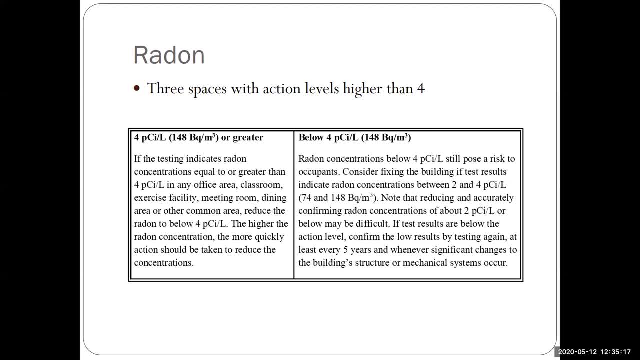 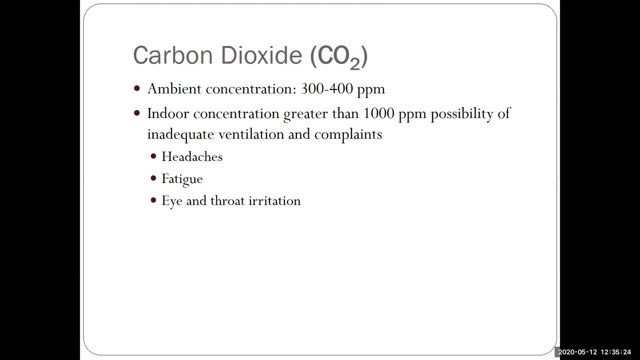 level, and we had three spaces higher than that. Our ambient concentrations of carbon dioxide were 300 to 400 parts per million. The indoor concentration was greater than 1,000 parts per million in some of the rooms at given points of the day, and so when we see that, we know that. 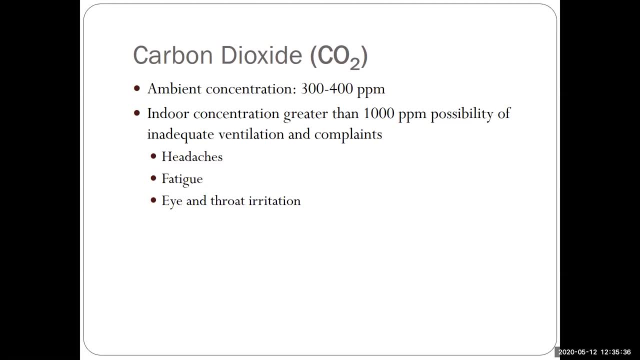 there's a possibility of inadequate ventilation and it can lead to complaints. So we're going to see four picocuries per liter and that's going to be our action level, and we had three spaces that had action levels higher than four, and so we're going to see four picocuries per liter and we had three. 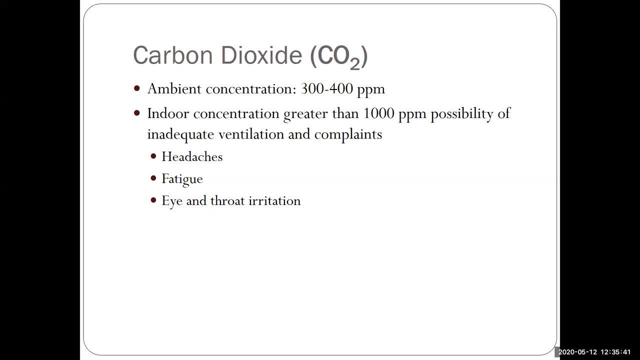 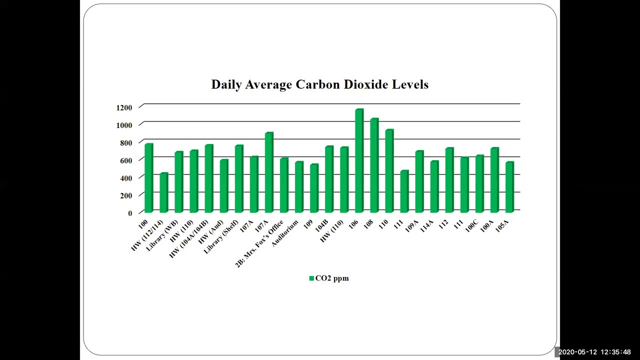 folks complaining with headaches, fatigue, eye and throat irritation. So in terms of the carbon dioxide levels, you can see these were the different spaces that we monitored. Each space was monitored all day long. so remember we had five different velocicals going. We would rotate. 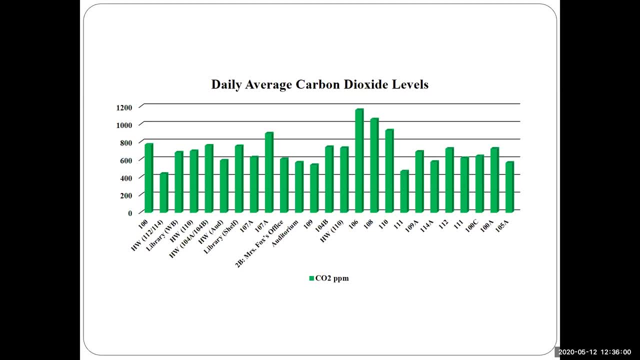 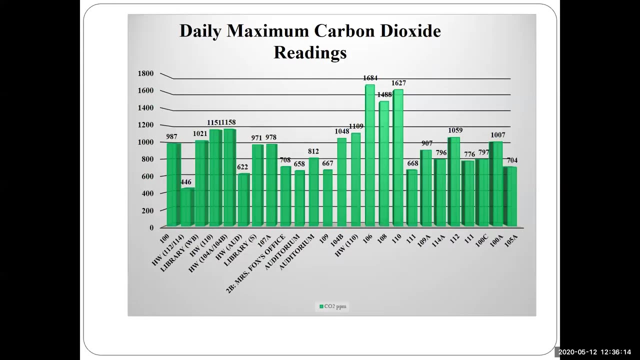 them each day, and so you can see that certain places we had peak levels, like room 106,, which was a classroom, went well above the 1,000 parts per million of CO2, and several other were peaking up above that If you look at the maximum carbon dioxide readings. so the slide. 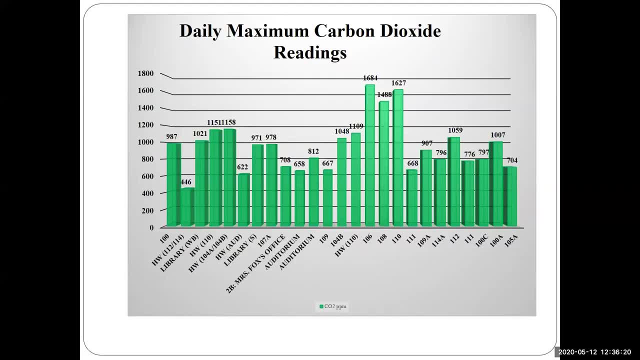 before was looking at your average. If you look at maximum, so for 106, when we saw that higher average, you'll see that it peaked out at 1,684.. The building has an occupancy of less than 20 for approximately one hour after the morning sessions, which means that after the students in the morning, 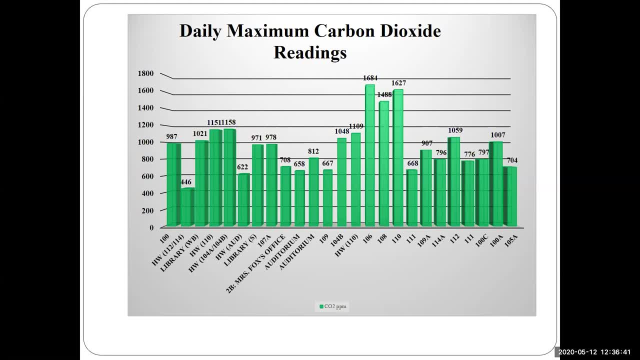 session leave. there's only about 20 people there, and those are the teachers and that's the staff, and it still took probably a good hour or more for these numbers to come down, and what's unfortunate is, by the time they start coming down, the afternoon session starts coming in, and so you're. 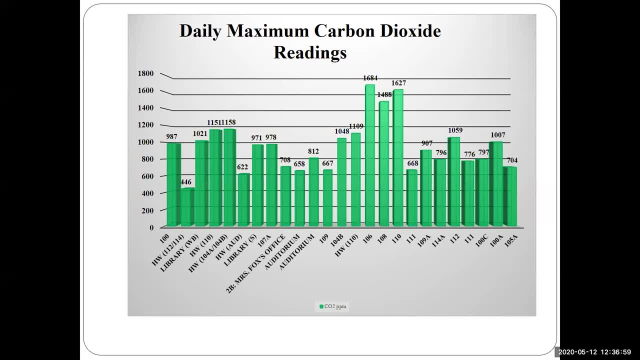 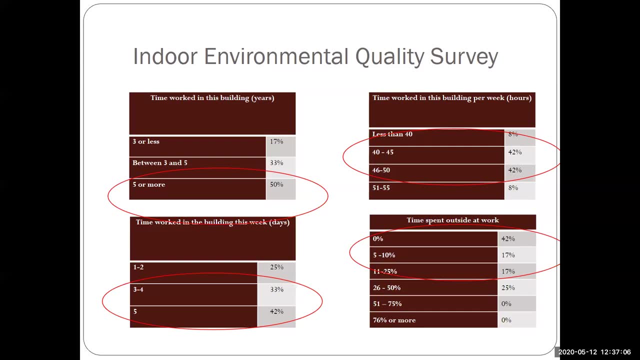 just going to see those levels go back up and then stay at those higher levels for over an hour or more after the school day has ended Now. so that was all the stuff that we monitored. Like I told you at the beginning, we did an indoor environmental quality survey so that we 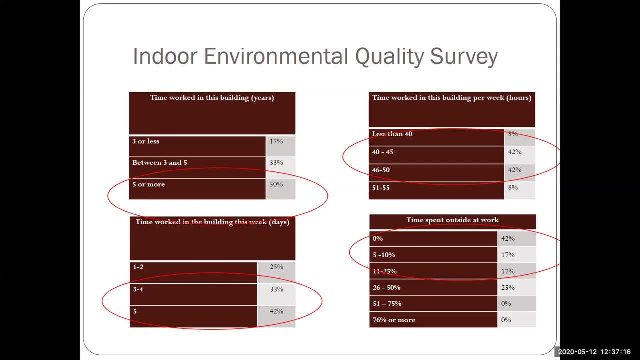 could let the teachers have a voice in this process. and so, if you look at our survey, time worked in this building in years five or more, so some of the folks had spent the good majority of the building's- I guess duration of existence- working in that building. okay, and they were. 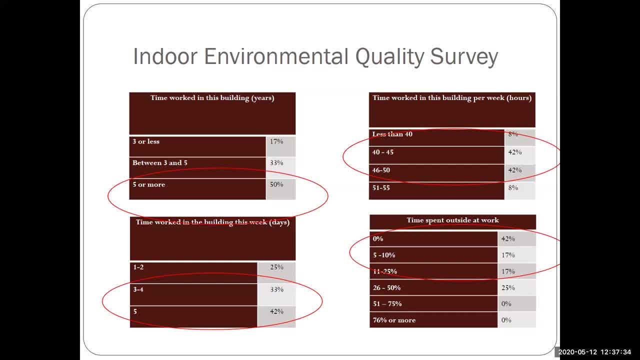 the ones that essentially were the most vocal about their symptoms and associating it with indoor air quality. Time worked in the building this week and days, so the majority of them were going to be working all five days. as you'd expect for the teachers, Some only worked. 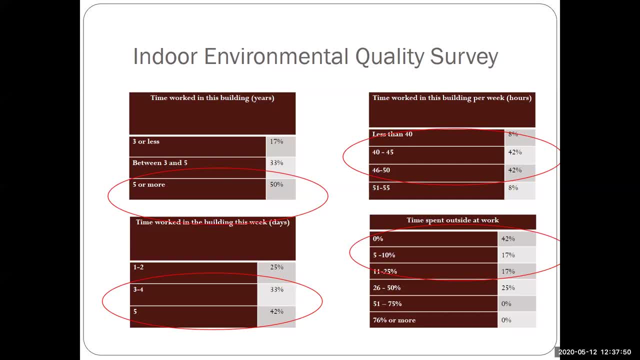 three to four days. It was based on their contract, so if they weren't teaching agriculture and they were teaching subjects such as English, math, the different sciences, biology and chemistry, they may only be there a portion of the week or a portion of the day, depending on what they teach. 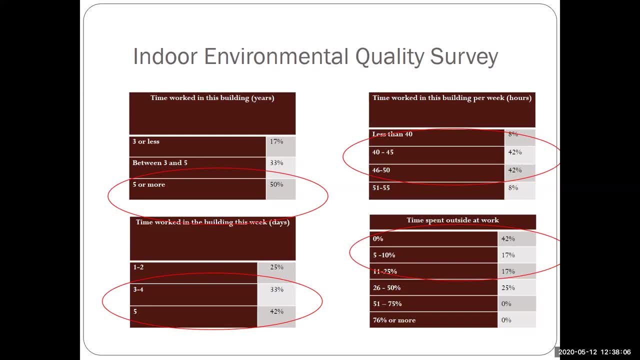 Time worked in the building per week this week and hours. so just to give you a little bit of an idea of what we're doing here we're going to be working, just in case you didn't know this already. Teachers put a lot of time into your students. 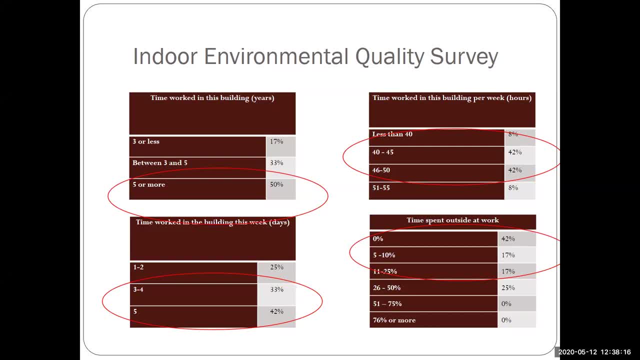 so the majority of them were there between 40 to 50 hours per week, so they're spending a good chunk of time at school, Time spent outside at work. Remember, this is an agricultural school, so we would expect that there would be a good percent of time spent outside dealing with the 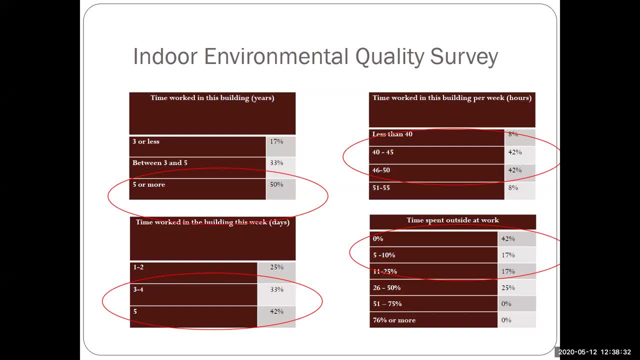 horses, cattle and other pieces of the farm. so 26 to 50 percent of the time 25 percent of the faculty were outside. Forty-two percent spent zero percent of their time outside. Remember, we have that vet tech program. 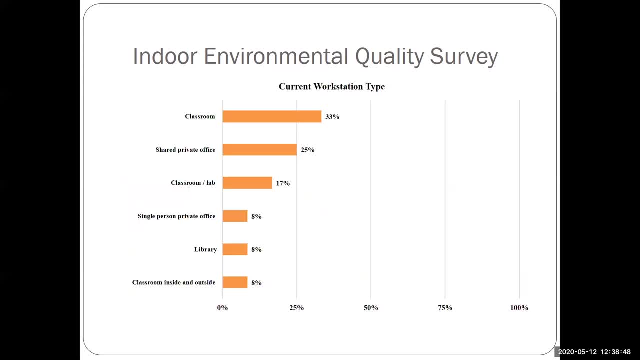 We have the traditional subjects being taught. This isn't surprising. Indoor environmental quality survey, their current workstation type- 33 percent were in a classroom. We had some that had a shared private office so they could be counselors, librarians or media. 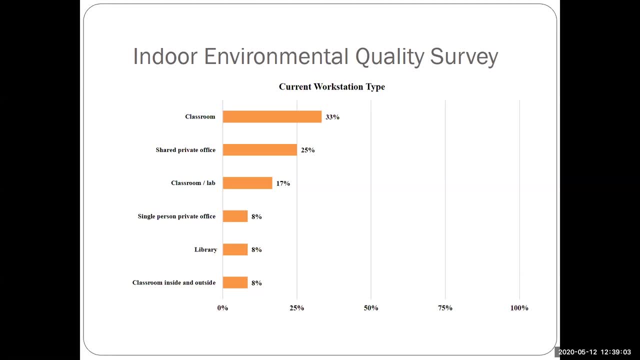 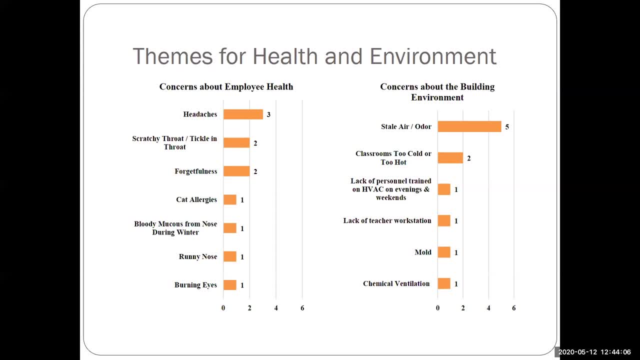 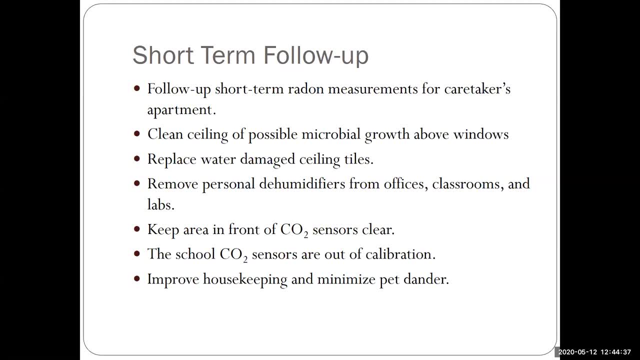 ceilings that we looked at Replace water damage ceiling tiles. In those tiles we didn't see microbial growth, the ones that were a closer up picture that we could actually capture with our phones. But what we were thinking is: you have uncontrolled water leakage. you could potentially 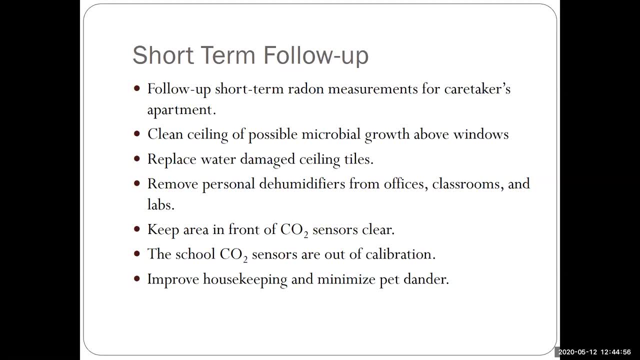 have fungal growth. Remove personal dehumidifiers from offices, classrooms and labs, Because recall that the relative humidity was well under 40. So you can start seeing issues with dry eyes and throats and that sort of thing, Keeping the areas in front of the CO2 sensors clear. So in many of 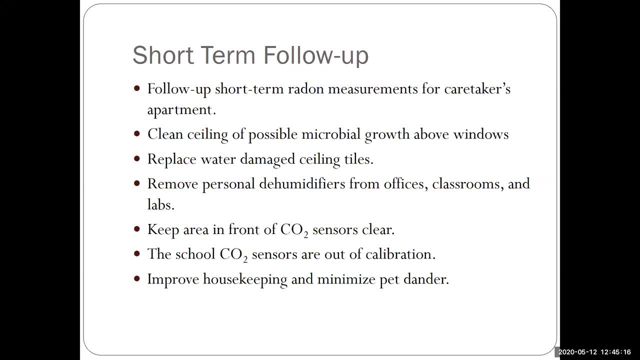 the classrooms, we observed that their CO2 sensors, which were built into the system- it's so amazing that they have them- were actually being blocked, So the sensor couldn't actually do its job. The other piece was- they admittedly told us the CO2 sensors were out of calibration, So the data that 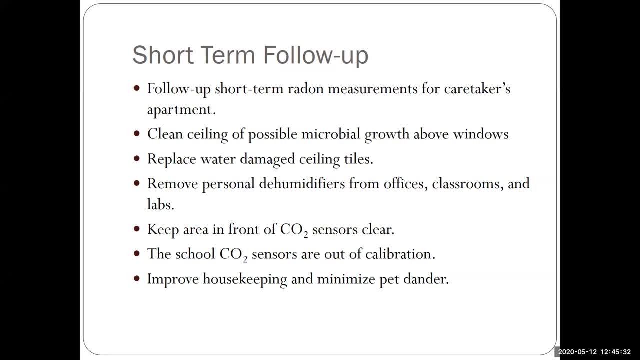 were being pulled out of the system. the data that was being pulled out of the system, the data that was being pulled and being sent to the central office for the school district, could not be interpreted appropriately because all the sensors weren't calibrated And the person who knew how to 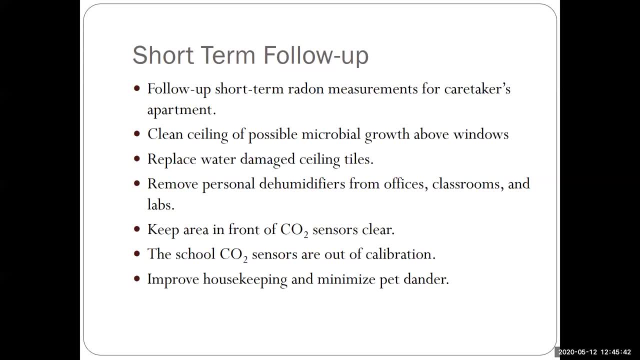 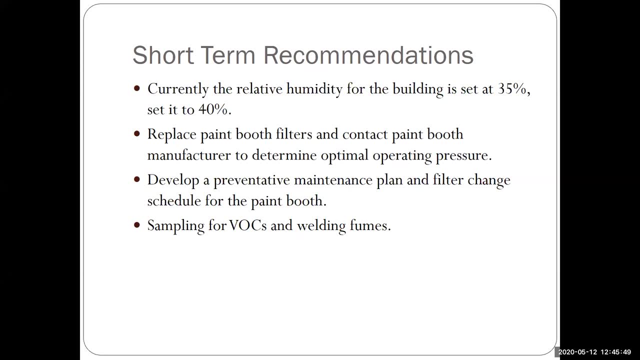 calibrate them had actually retired. And then, of course, improve housekeeping and minimize pet dander. Other short-term recommendations, you know: replace the paint booth filters. contact the paint booth manufacturer to determine the optimal operating pressure to ensure that they're. 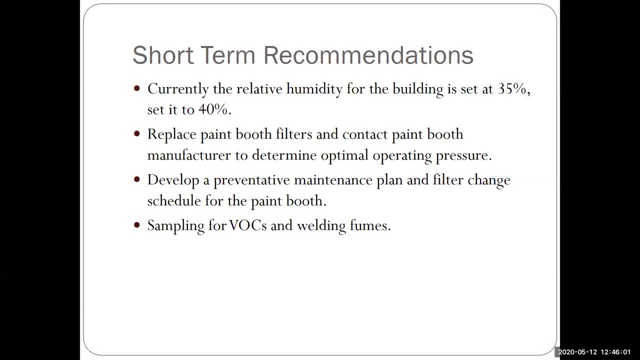 protecting those students who are learning a skill to one day work in the field. Develop a preventative maintenance plan so that that type of filter disregard wouldn't happen again in the future, And just putting it on a schedule so someone knows to change the filters after a good 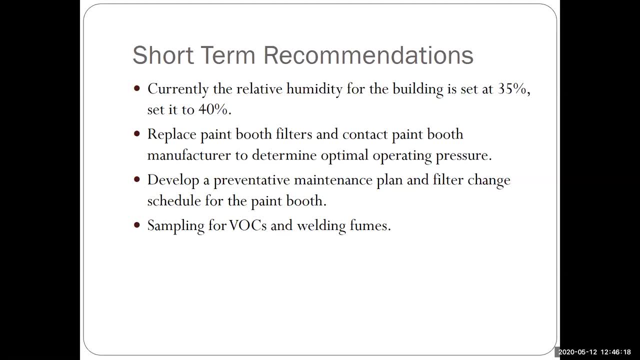 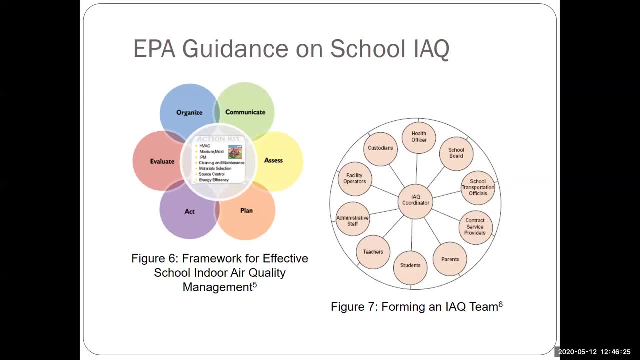 percentage used And then sampling for VOCs and welding fumes, because we just did not think that the ventilation they did have was appropriate. One of the other items that we told them that we thought would be a good thing for them was that they were going to be able to use the filter. 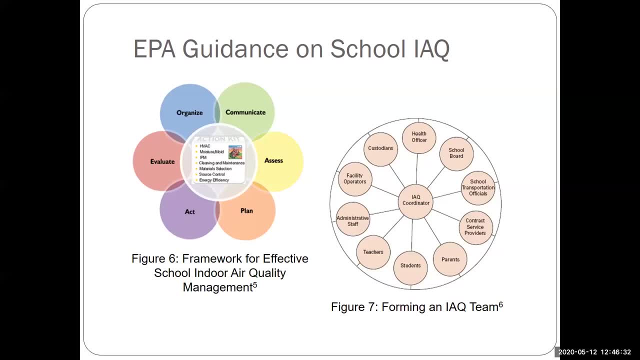 they had. This was the first time we were able to do this, because we didn't know what the fluid quality would be. So we did get some feedback on, you know, the quality of the filter that they needed And we decided that at this point you know we're going to have to do it again, So you 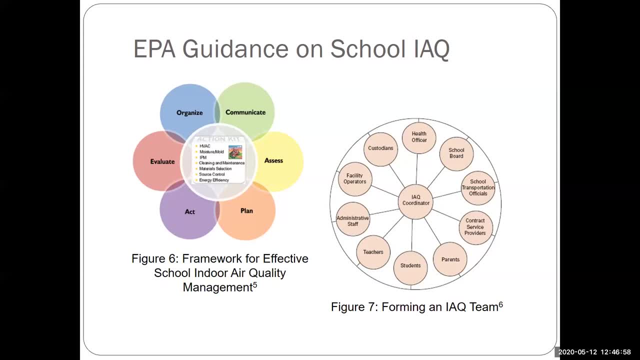 know it's a wonderful thing, And the last thing we wanted to talk about, since we're not going to talk same things. we looked at the HVAC: looking for moisture or mold, thinking about their integrated pest management so they have less of those biofluent issues. cleaning and maintenance. 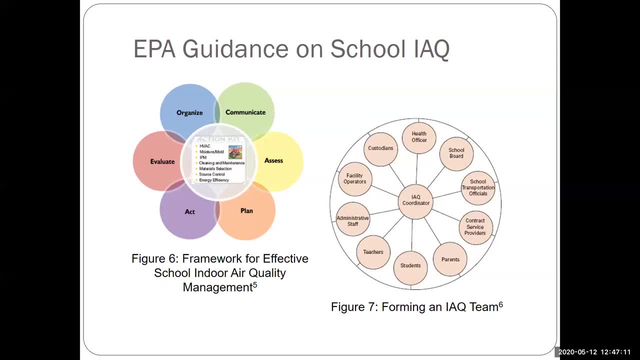 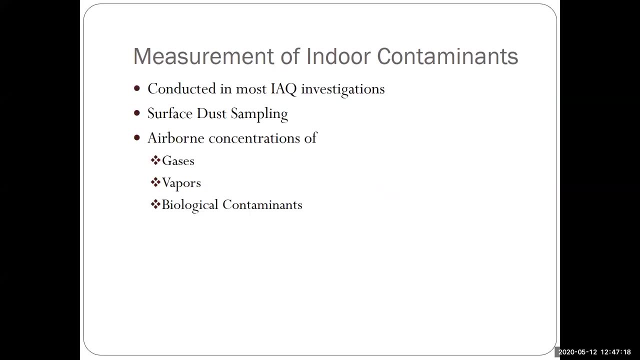 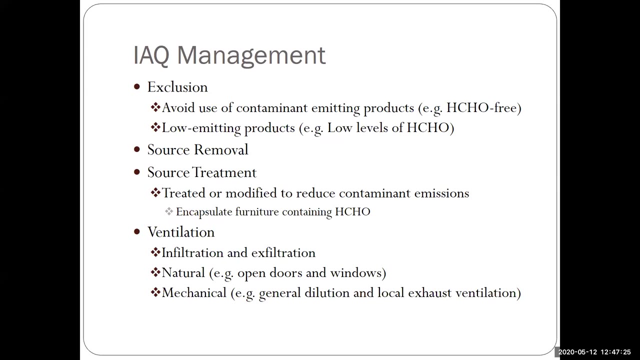 schedules, the materials they're bringing into the building, the sources of some of their issues which were in their classrooms- They could have closed things off, capped things off- and then also their energy efficiency. right, I want to go through two last slides before we end. 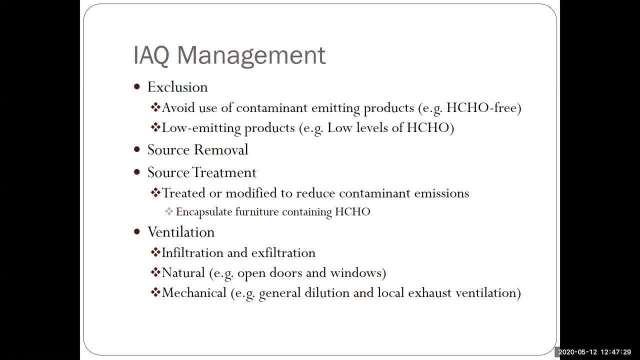 just so I can end on time and give you guys a little time to ask questions. When we think about IQ management, exclusion, obviously, is where we want to go right. Exclusion: We want to avoid the use of contaminant emitting products when we can. but I came from industry and I know that. 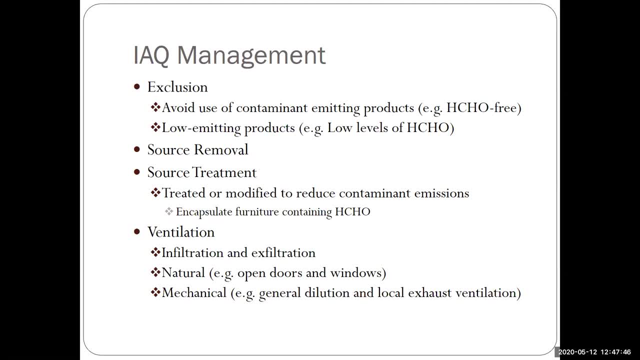 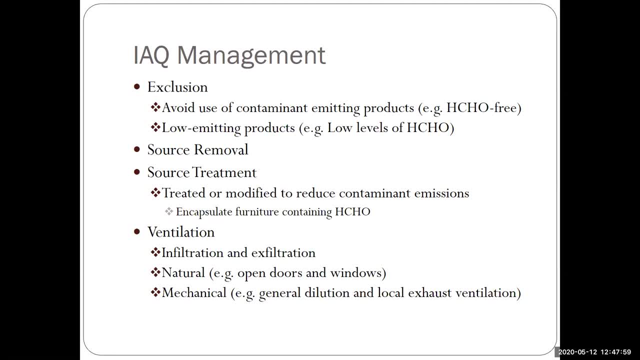 for you. I also know that sometimes it just depends on what you're budgeted right. If you think of a school district, they have a very finite budget and a lot of things that they need to actually provide money to, so they may not be able to do that Switch to a low-emitting. 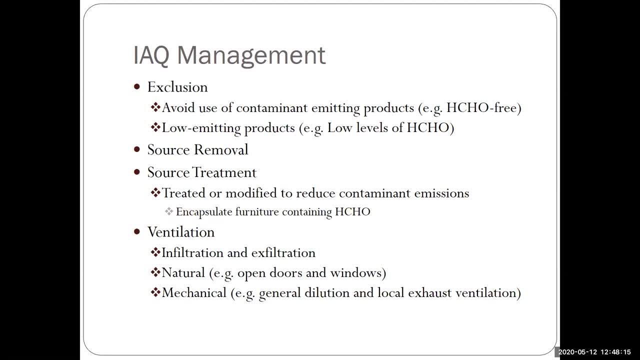 product. So if you can't avoid the use of that contaminant emitting product, get a low-emitting product. Source removal. you know, take the source out if you can. You can also source treats. So if you know that your furniture, for example, 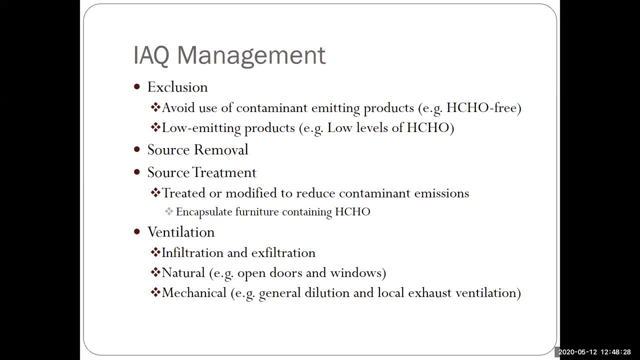 is going to have issues with formaldehyde. is there something you can purchase to encapsulate it, some sort of treatment, Ventilation? Look for infiltration and exfiltration of your building. Where are things coming in and going out where they should not be right? Find a way to seal. 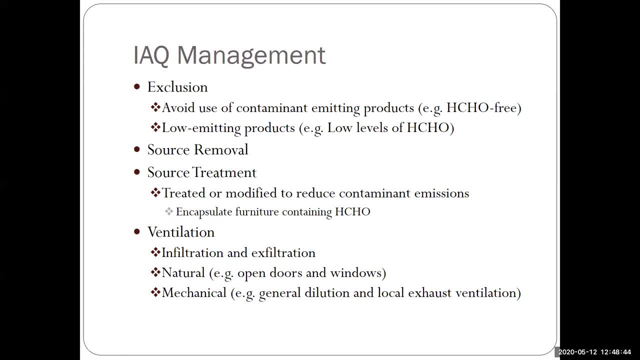 those And then thinking about natural. So natural ventilation would have been good for some of those rooms had they had more control over their windows. But with natural ventilation, we know, comes other issues, because then you have all those ambient air quality issues. So if you have 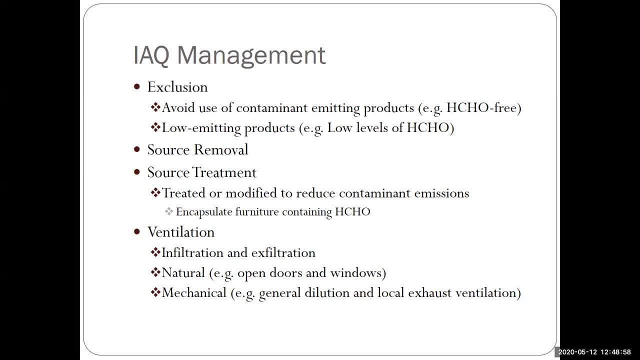 those ambient air pollutants that could then come into that indoor space. So it's a trade-off. And then mechanical, So thinking about the general dilution of the building. So take, for example, the hallways in the school didn't have ventilation. Also think about local exhaust ventilation. Why? 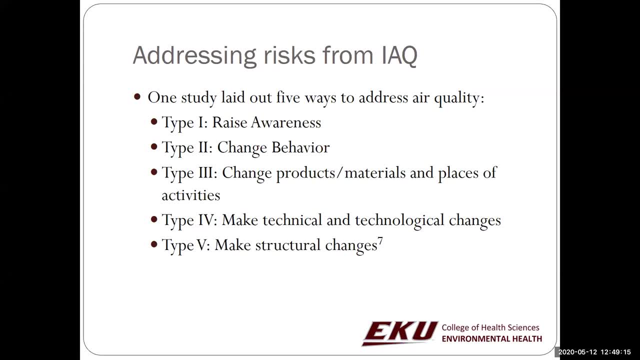 have it if it's not going to do the job. And then the last slide is just thinking about addressing risk from an IQ standpoint, almost like a hierarchy of control. So five different ways I found in the study. Type one is just raising awareness. So when you go in to do an IQ study, educating folks on 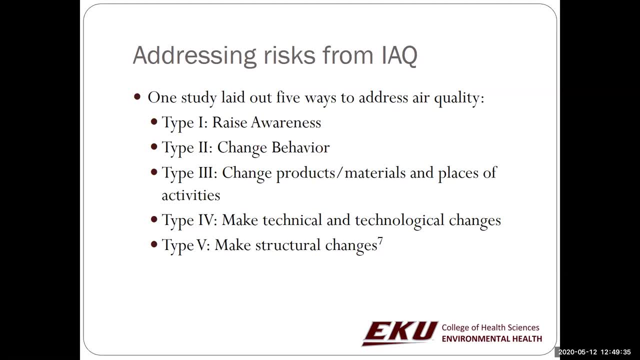 hygiene. What's appropriate with chemical use? What's appropriate storage use? What's material handling look like for them? Talk to them about the characteristics of their cleaning products. Go over the safety data sheets with them. They may not even know what a safety data sheet is. 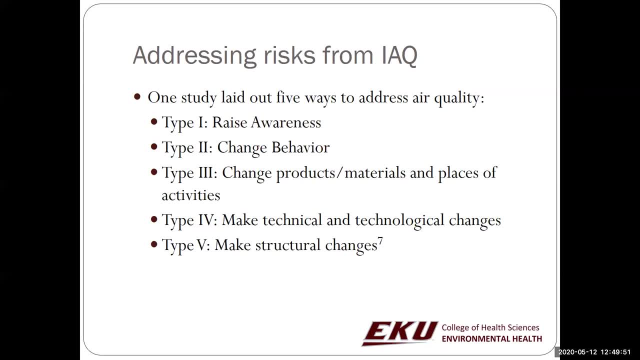 Sheet is They should right Because of Hascom, But maybe they don't. Maybe they just kind of browse through the training that day, Thinking about changing the way you're cleaning. So changing behaviors, right. So getting folks to improve their cleaning actions. So cleaning more. 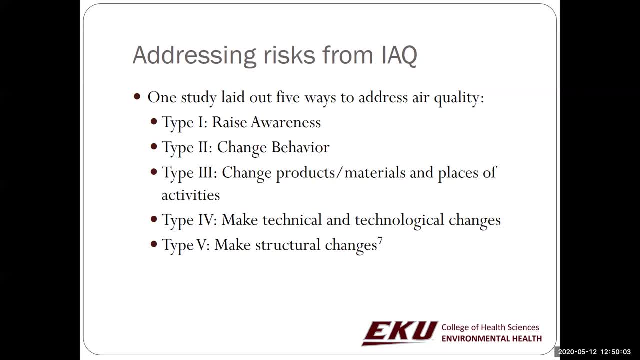 to reduce particulates in the air, But then also thinking about the products and materials and the places of activities. right, The type three way of addressing air quality. Type three: we could use a vacuum instead of a broom. So the vacuum is actually capturing the dust and the broom is just knocking. 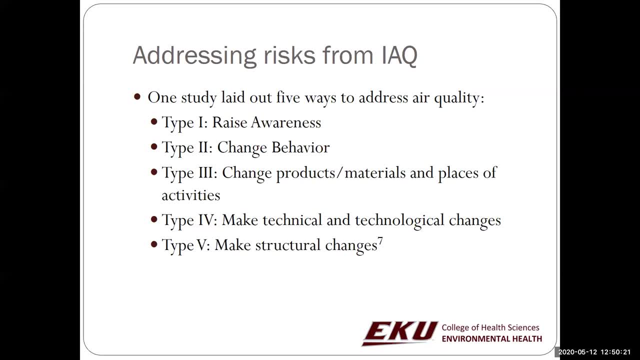 it into the air, re-suspending it for you to breathe in. Use different rooms based on the type of activity to be careful about. So if you're doing a cleaning action, you're going to want to be careful about that. So if you're doing a cleaning action, you're going to want to be careful about. 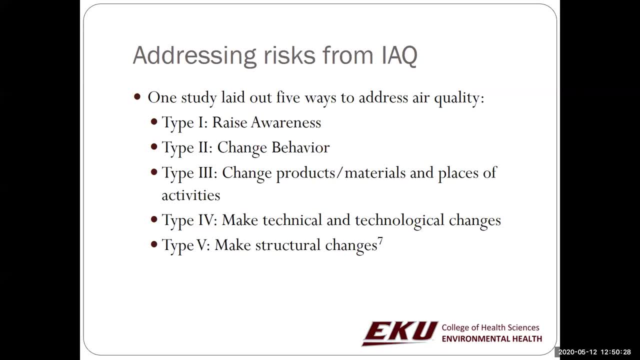 it out, Point in case: don't do diesel mechanics in a room that was built for equine type work, working with horses, And if you are, you need to think about the ventilation right, You may have to change that. So, type four: make technical and technological changes right. Put in the type of 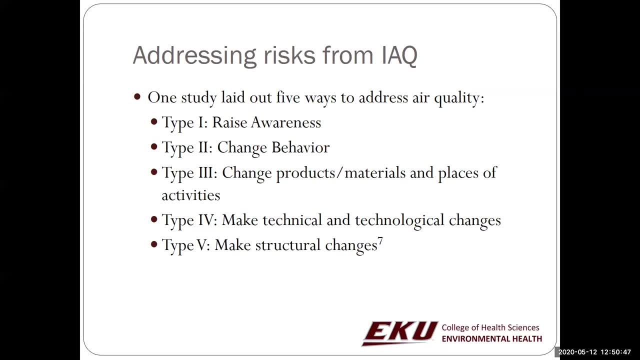 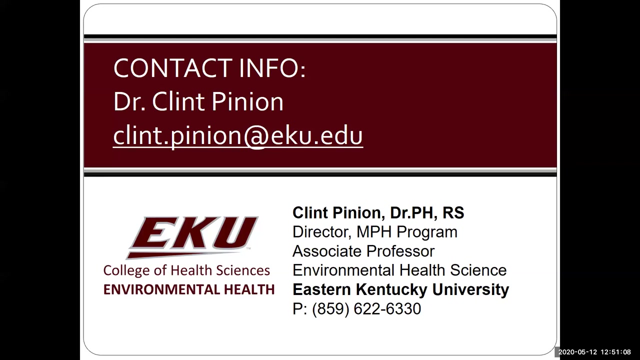 ventilation you need for that room. Type five examples: This is structural changes. So instead of using chalkboards, use whiteboards. Instead of using whiteboards, use the overhead projector with the monitor and take out markers and take out chalk. And this brings me to the end of my presentation. This is my contact information. Again, I'm Clint Pinion. 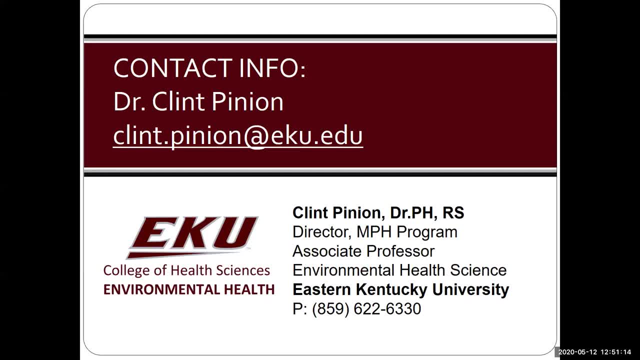 and I work at Eastern Kentucky University And any time you want to drop a line, I would be happy to receive your emails at clintpinion at EKUedu. Thank you so much for that excellent presentation And I'm going to turn it over to you. 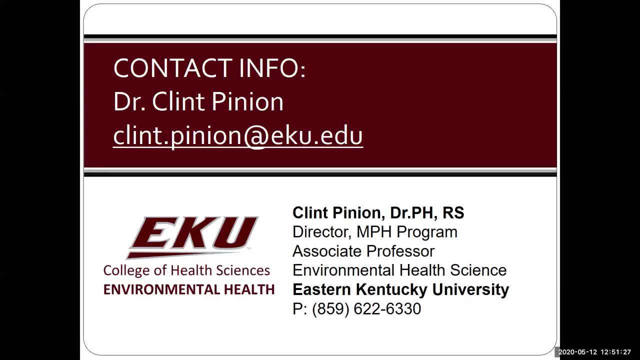 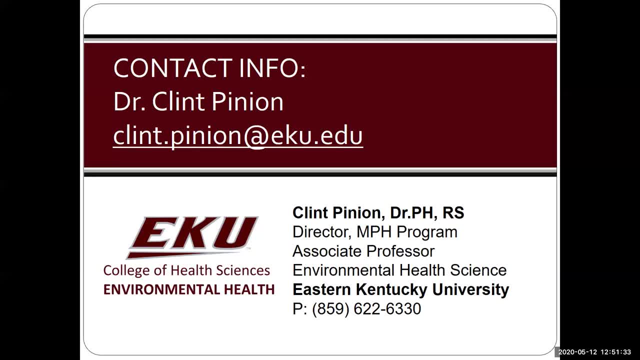 enter any questions that you might have into the Q&A box And I'm happy to read them aloud. Our first question: someone was wondering if the teachers and staff were asked about time factors, like what time of day, where and when they experienced issues with the indoor air quality. 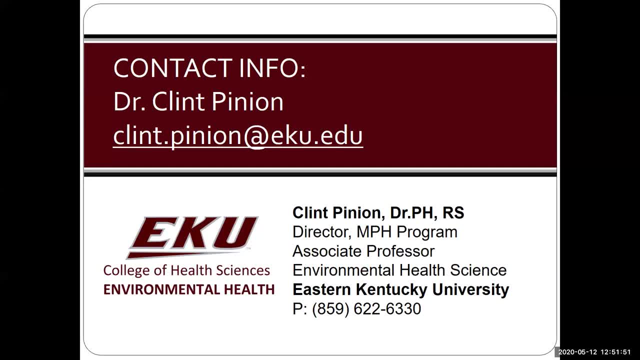 So we did ask them and we met with a lot of the teachers like one-on-one. I wouldn't call it like interviews, if you will Like, we would think about in the academic world, But we did meet with them kind of informally And what they told us was, as the day progressed, especially in classrooms where they've been teaching all day, that's where they would start to experience the headaches, the fatigue. 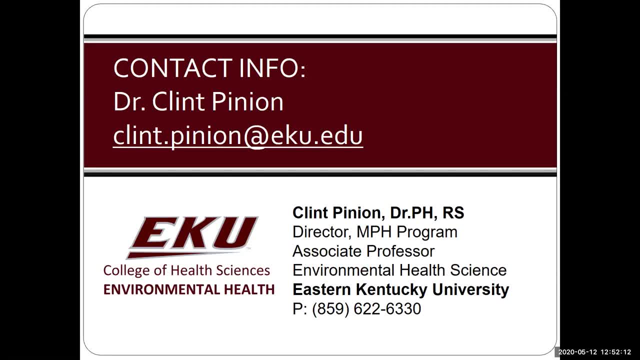 So we did ask them, but we did not ask them with a survey. That would have been something that would have boosted the survey. The other thing is, of course, like with the diesel mechanics: as the day went on, that particular teacher noticed more headaches, But again he had been working with the students. 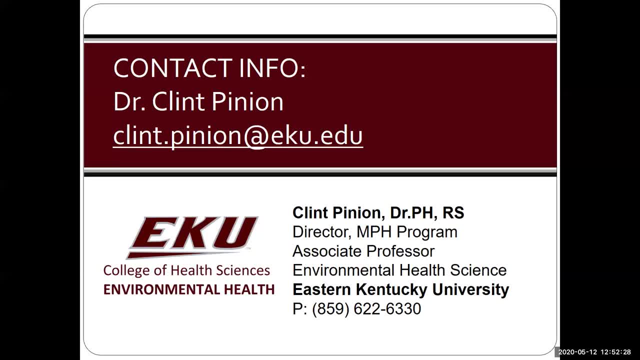 So we did ask them and we met with them. So I think that's another question, Yeah, and we also looked at the use of the classroom discussion and how they answered those questions and shared thoughts and comments, and I think one of the things that's really great about the Q&A is that it's a really good way to give feedback as to the other participants. 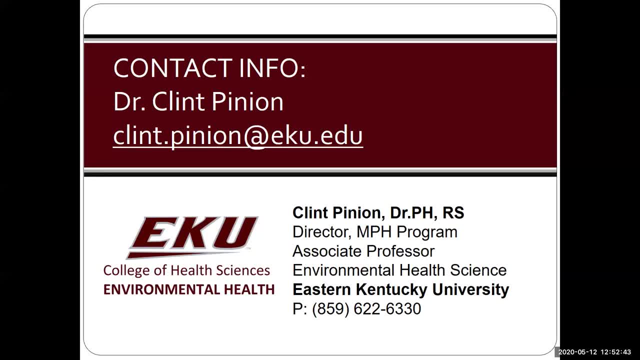 So it's really important to have these conversations because this is where we talk about what to do. maybe technical staff, maybe other participation is important, or maybe not, But there are tools around all those different chemicals and oils and fuels and whatnot throughout the day. So usually towards the end of the day, which is what we would expect, especially with comfort parameters, with CO2 and CO0 and the temperature issues, we would expect that, as there's been a lot of bodies in and out of those classrooms and labs, 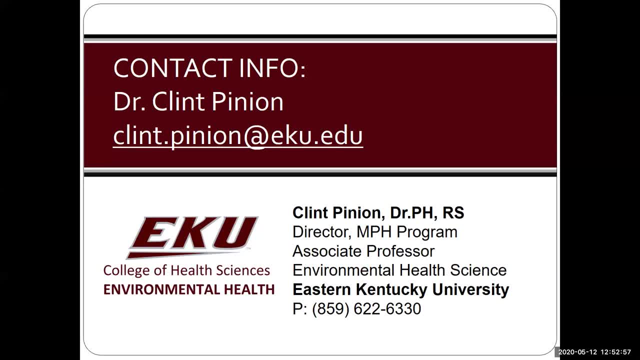 Thank you. being a consulting type approach, we gave them short-term, long-term recommendations and then, of course, we told them we could do a follow-up and help them implement. we were not contacted back. i think it may have gone back to that over time. they'd had so many iq issues they felt like many. 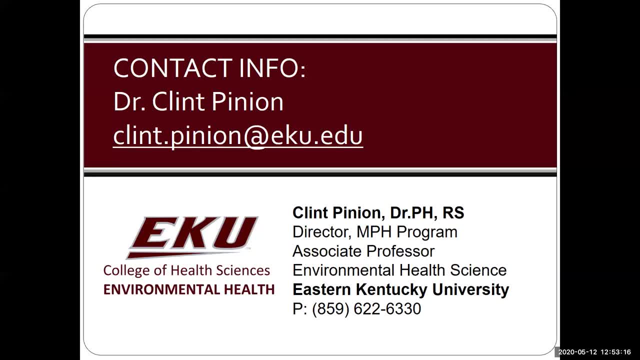 of the things were easily addressed with our short-term recommendations and they didn't follow up with us. we did contact them, um, i think it was actually earlier this year and they didn't have any updates to provide. great thank you. and if there were any previous consultant reports were. 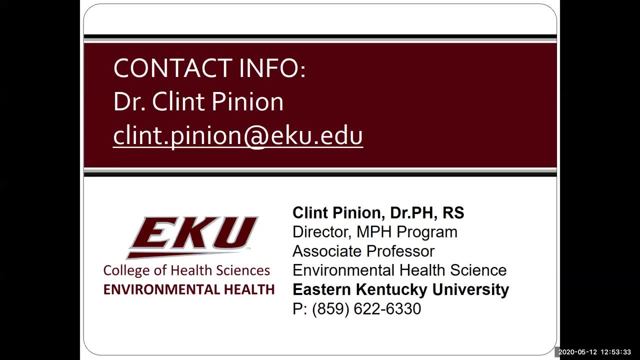 you given the option to review those. we actually were. we were fortunate enough to see the past work, so we had excel sheets that included the data of any of the monitoring that had been done. so if you think about the radon and comfort parameters, we could see past studies that had been done at. 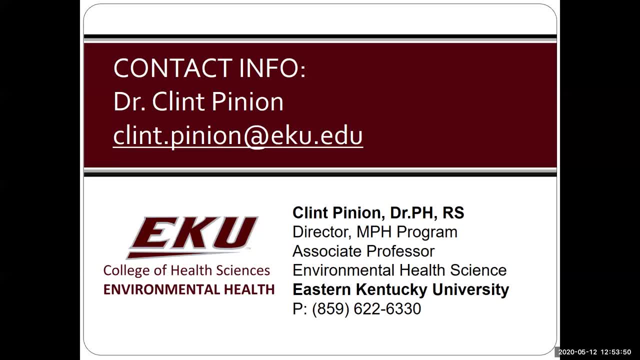 the site and so in the past it was kind of what we were seeing. you would see peaks with co2 and co at certain point-of-life and in the around time we have seen a lot of people working on some of the tasks that lie in the field, like: look at the data that we're looking at right now, how many people 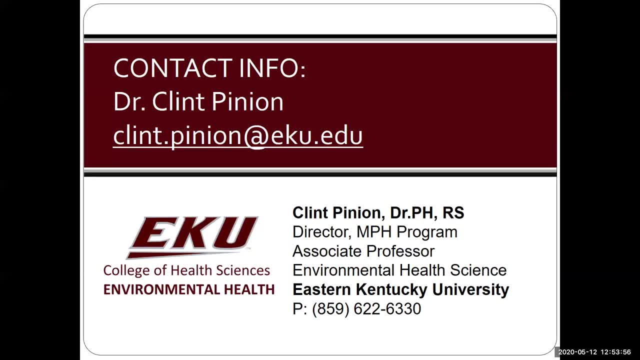 points of the day. They did have some early on issues with radon, but that was corrected Again. they had a radon monitoring system which helped them stay on top of that And, of course, the school could use their ventilation to their advantage to bring down radon levels. 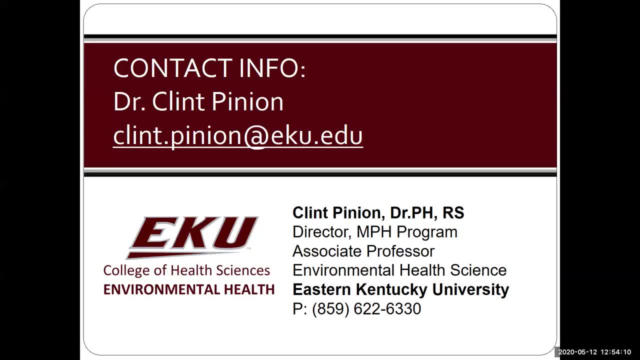 Great thank you. Regarding compliance and relevant standards involved with indoor air quality, this person has a question about OSHA, So assume OSHA would have jurisdiction over the building, as the faculty and staff are employed at the school. However, are there any other regulating? 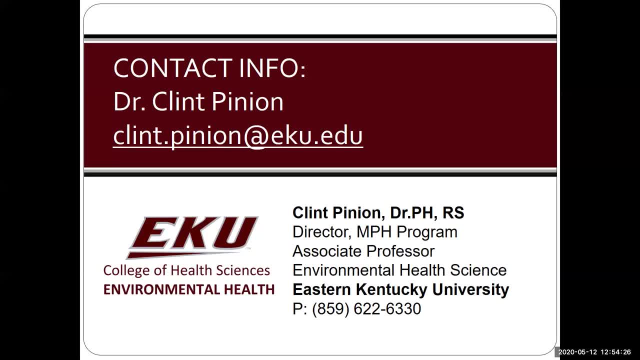 bodies that ensure safety standards are met for the sake of the children at the school. Yes, so one of the things that comes into play because you have to think about local municipalities- health department can come into play And, quite frankly, I've given an IHQ. 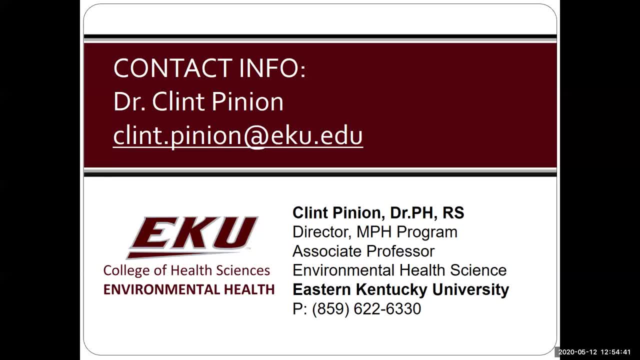 presentation at one of my local environmental health association conferences and it came up again and again and again because the health department's environmentalist get called out to the schools because of the endangerment of the children. Like it gets brought up. oh, my student says that they're having headaches while at school. they can't. 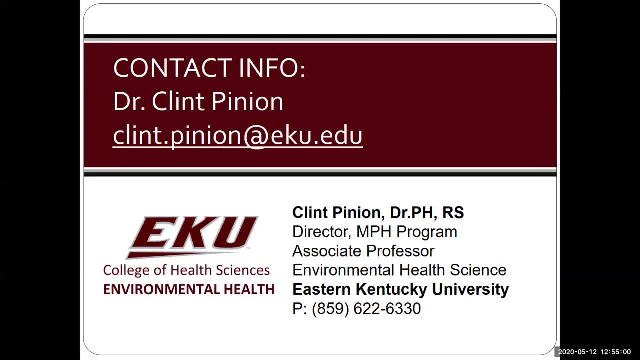 focus. So the health department gets called, And so then the health department has to go out and they have to do their own investigation. Many times they aren't exactly trained in IHQ issues. A lot of their work is geared more toward sanitation, dealing with like water, wastewater, 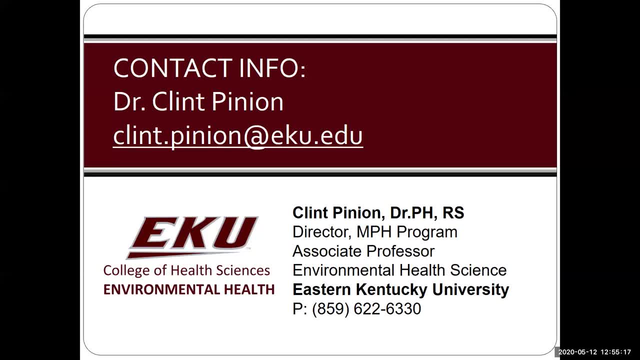 food issues And then, if you think of their air quality, they do a lot with, like EPA's implementation of the ambient air quality standards, So they came into play. So that was one of the the only other agency that we had information that had been out. 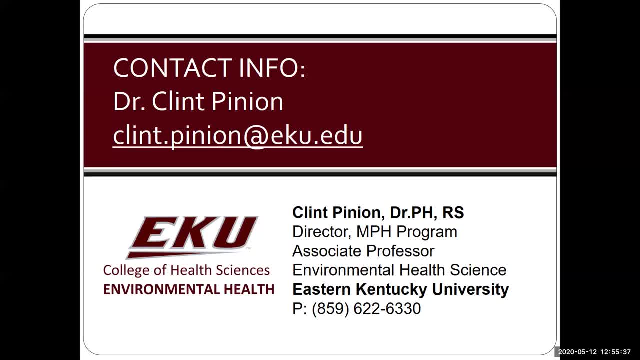 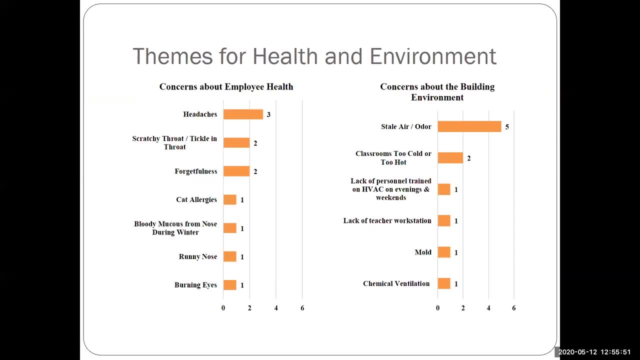 to do a study. Excellent, Thank you. And how do you go about IHQ assessments where an industrial hygienist, for example, has no idea on what's occurring, one that may seem like an unsolvable puzzle? If you don't mind, I'll go back to my slide. Sorry, folks, look away from the screen if it's. 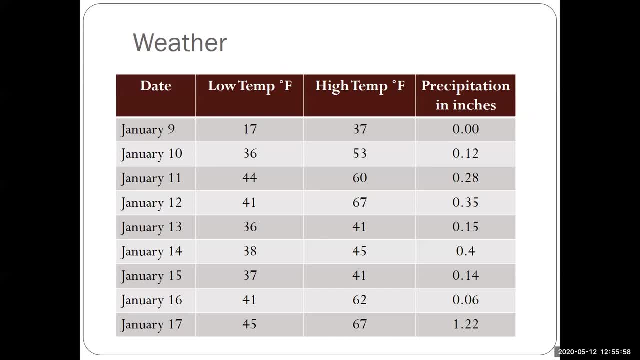 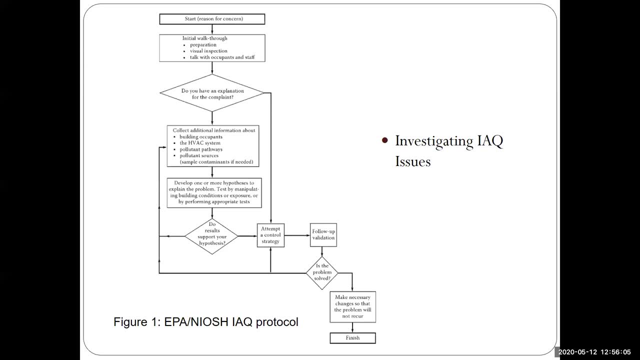 going to cause you any issues. But going back to this diagram, this flowchart, it's really good because you make your assumptions based on the data you have. You test that assumption. If it didn't give you the- you know basically the outcome you expected, you go back through the 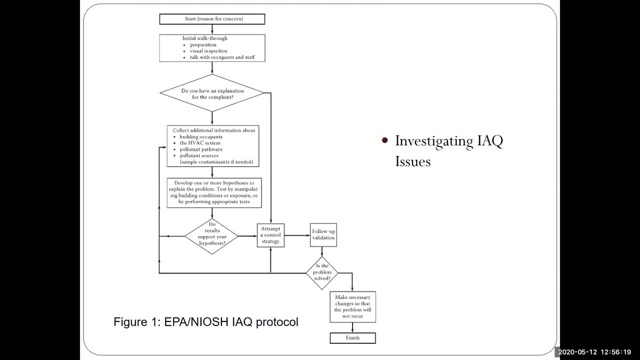 process and try to figure out: where do I need to get my data from. And then you go back to the question: where do I need to get data from? With whom do I need to speak, you know, to figure out how I get HVAC system diagrams, How do I get access to the school at different periods of the day, How. 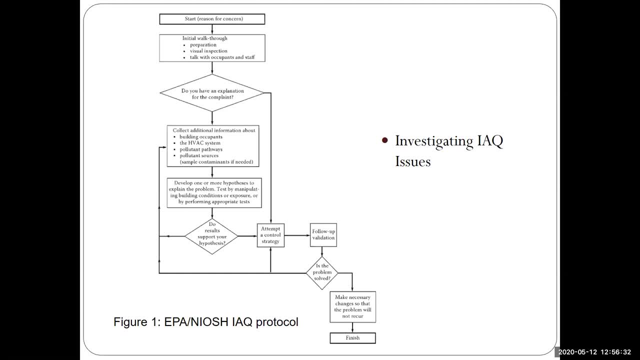 do I get access to the inhabitants of the building? So it really is most of the time trial and error. I don't think anyone goes in knowing exactly what an issue is, But over time if you see the same type of issues from similar buildings, there may be some commonalities. But I think each building 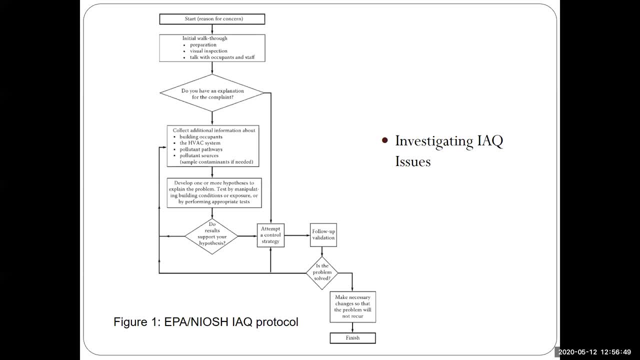 is its own beast And you have to take this diagram And your own approach as a professional and go back through and just adjust based on what you find. Thank you, And would you recommend an IAQ coordinator to all school districts, And how do? 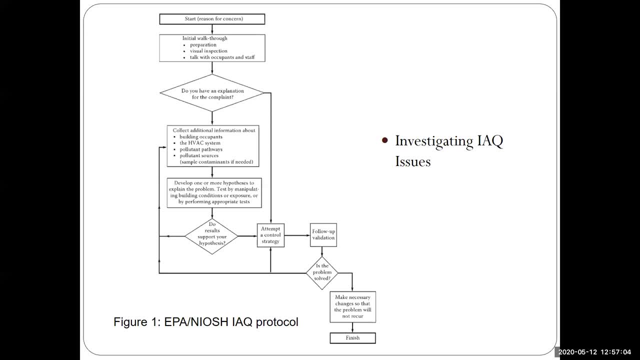 you foresee that taking place? Of course I would. I mean as an environmental, occupational health person. I think having someone at the school that is the face of indoor air quality issues would be a great thing to have, But I'm realistic in the approach that most schools 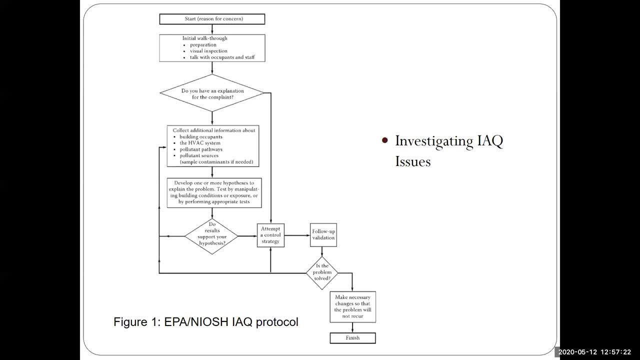 because they are so busy. I mean, if you think about what we put on our teachers across the nation, we put the education of our young folks in their hands and they have to take care of that, Plus all that comes along with it, right, All of those interpersonal issues. I doubt that IAQ is. 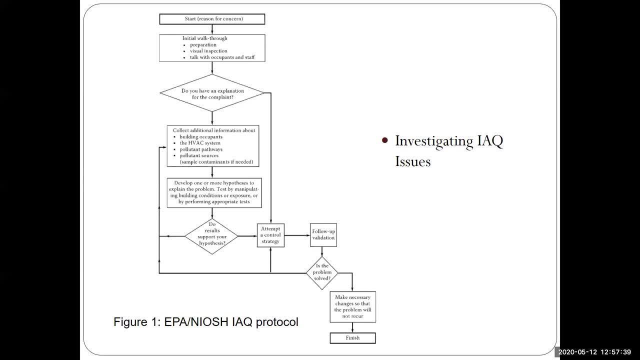 going to rank high on their list, And so I would love to see it, but I just don't think that you could require it right. You could recommend it, which is, of course, what is recommended by the EPA, But it would be so difficult to roll out. 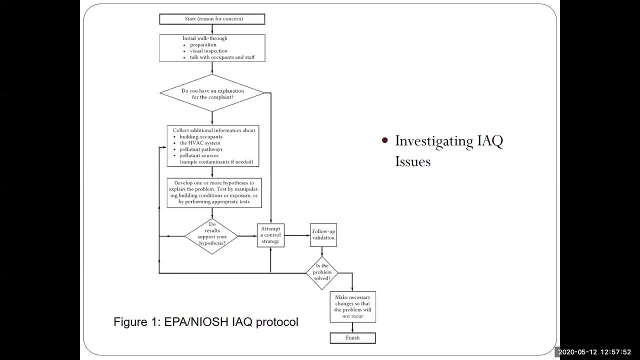 I mean it would almost have to be a mandate from the state board of education, which I doubt would happen, just with all the issues they have to deal with each day. Thank you, And in these types of projects, is there any resistance from the client or from other groups of people regarding? 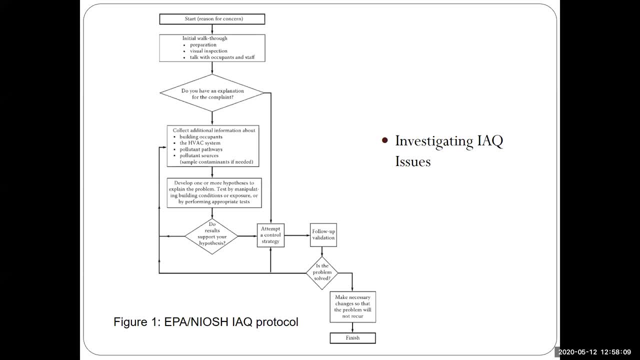 the data or the solutions that you come to. Oh, of course, I think when you have folks who feel there's an issue and you present the data to them and say this is what the data are saying, and it doesn't really matter, you can't do anything about it. And so I would love to see. 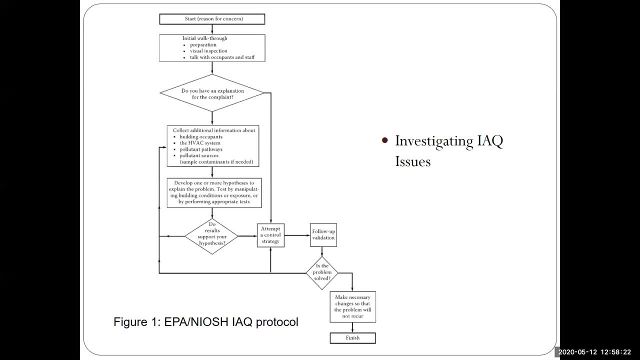 really turn out how they had anticipated, There's backlash. I mean, that's human nature. If you had it in your mind that something was going to be there when you get the data back and it wasn't, then you're going to be upset, And then there's the opposite end of that. If you were the folks. 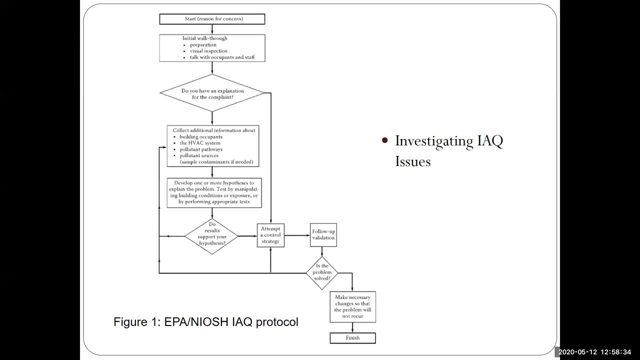 calling us in so that you could appease someone, right, Because sometimes IAQ issues it's also showing Like when we see the data. it helps us calm down a little that okay, we're in comfort parameters, We're okay on these numbers. They may not want to know that. yes, we did find things. 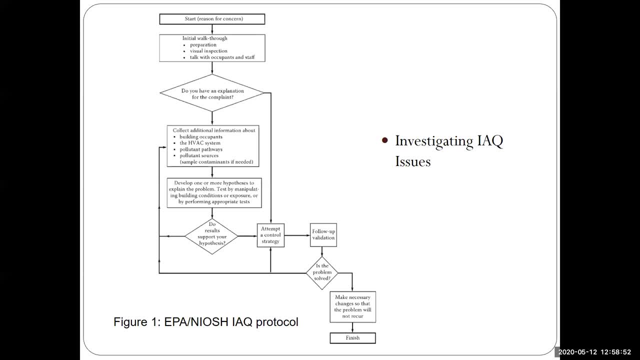 above action levels or, yes, we did see things that could be an issue for them. But you give them the data, you give them the facts in your report, you go over it with them to educate them, and then it's really on them to decide how they handle it. from that point moving forward, You can't make 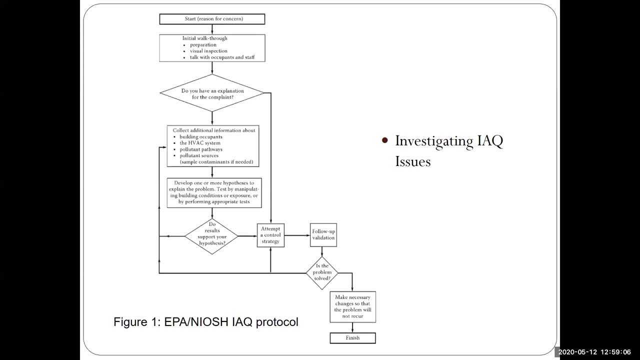 them do what they need to do. You are just a consultant giving your opinion based on your professional experience. Thank you, And we also have another comment slash question. ASHRAE reduced the CO2 guidance level from 700 parts per million above outdoor air by making it a flat 1,000 parts. 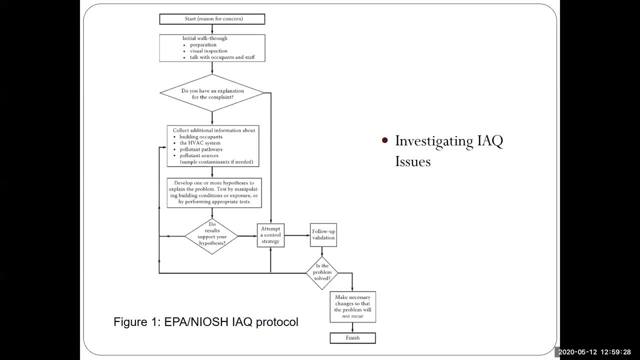 per million. I find complaints occurring around 800 parts per million and sometimes even lower. What is your opinion of these numbers? in predicting occupant discomfort, Well, I also find what you're finding, so I agree with you. I think it also depends from: 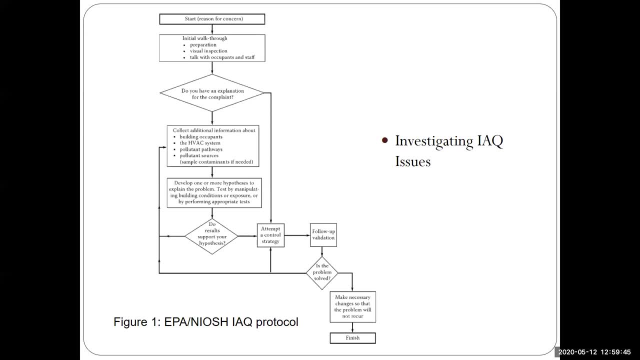 situation to situation. I think each person is so different- I'm talking about the people experiencing the IAQ issues- So sensitivity, just in general, to IAQ issues will make a difference. I think honestly that a lower number is probably going to be more representative of what's going on, just because the higher we 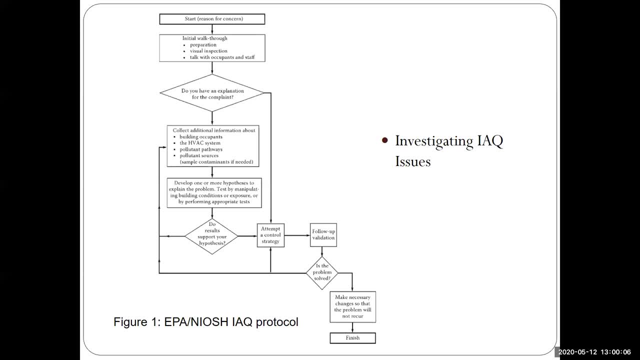 get it almost kind of discounts what that person is feeling. if that makes sense, Great. Well, thank you so much. We are coming to the close of our time here, but I did want to ask just one last question. In your experience, you've mentioned budget a couple of times in terms of maintenance. 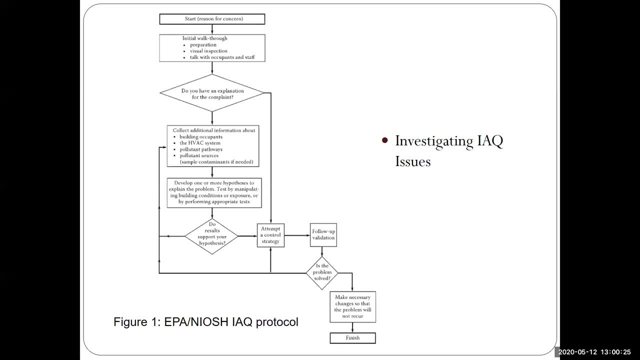 budget being considered discretionary, or the allocation of resources to lower emission products, substitutions and et cetera. Are you able to provide, I guess, any advice as to someone how they can communicate with a client about the benefits of allocating budget towards indoor air?